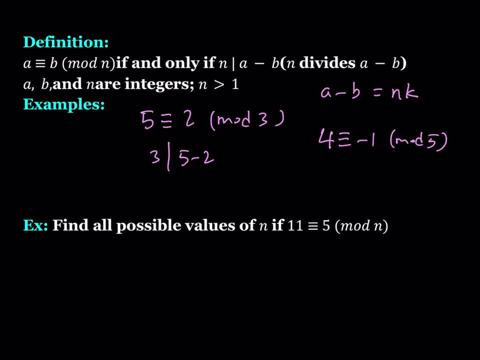 negative numbers as well. This is also true because, if you think about it, 5 divides 4 minus negative 1.. Here we have to be careful when subtracting a negative number. Okay, now let's take a look at this example. This is one of the first examples that I actually 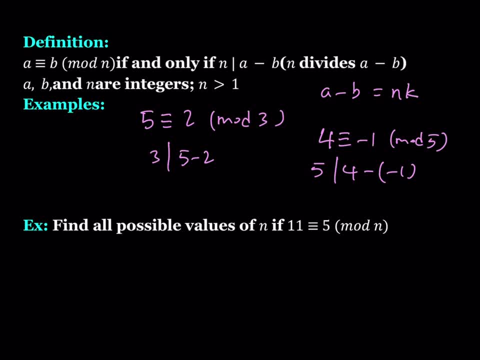 go over when I teach modular arithmetic. Find all possible values of n if 11 is congruent to, So that's how we read it. Congruent to 5 mod n. So in this case we don't know the modulus, we're trying to find it and we do know that. 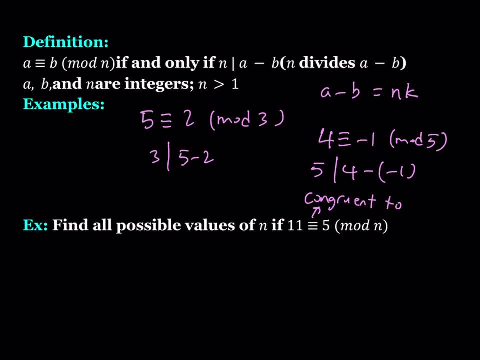 11 is always congruent to 5.소. we can use our formal definition. Basically, what it means is if a is congruent to 5 and 11 is congruent to 0. Now what we're going to do is look at these values, so we're going to 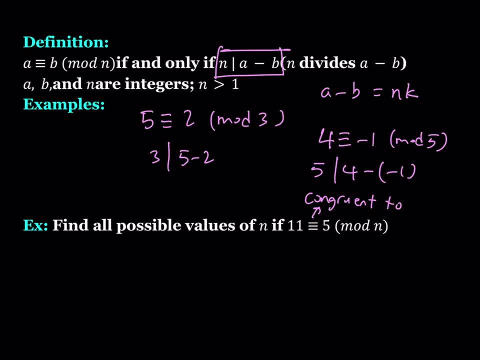 to b, mod n, then n divides a minus b. So we can safely say that n divides 11 minus 5, which means n divides 6.. And of course n needs to be greater than 1, and it's going to be an integer. So what? 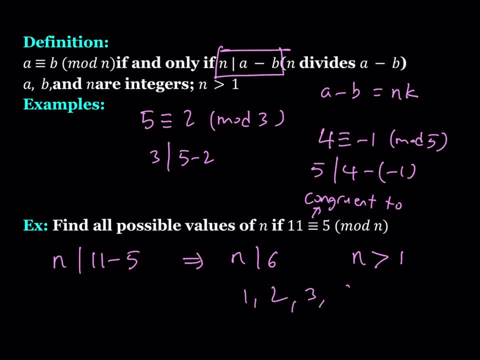 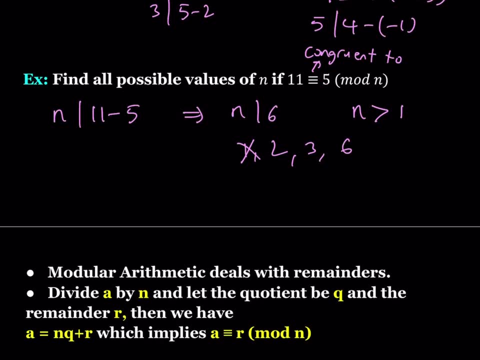 integers divide 6?? We have 1,, 2,, 3, and 6.. Since we're not going to count 1,, we have 2,, 3, and 6.. These are going to be the possible values of n. Okay, great, Now modular arithmetic. Why do we? 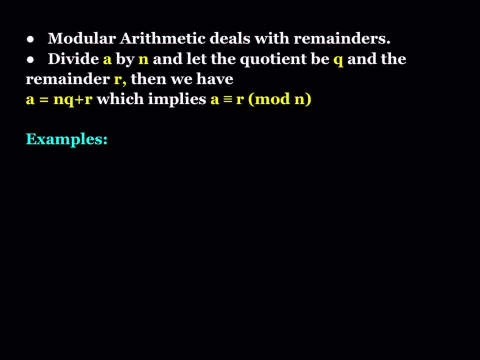 use modular arithmetic. It deals with remainders. So if you take a positive integer, a, and divide it by n, another positive integer, and let the quotient be q and the remainder r, then from division algorithm we can basically write the following, which implies a is congruent to r mod. 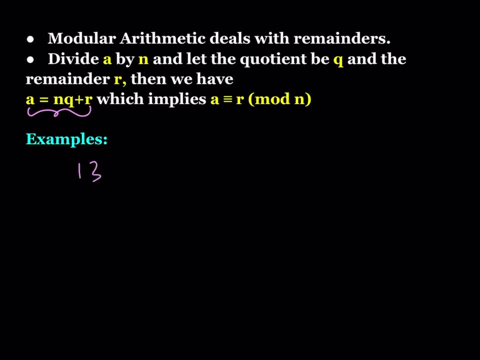 n. Let me go ahead and explain this with an example. So suppose you're dividing 13 by 5, right? Well, of course, when you divide it by 5, the quotient is going to be 2, and the remainder is going to be 3, right? 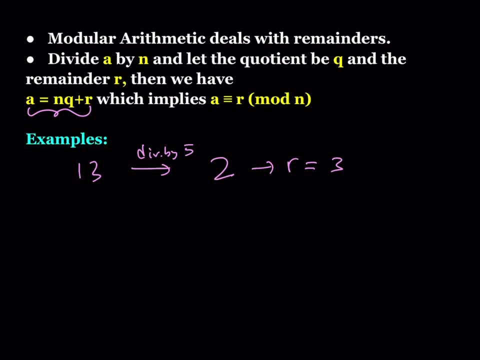 Okay. so what is that supposed to mean? It means that in this mod, which is mod 5, we're talking about mod 5 here because we're dividing by 5.. Remember, when you divide by n, you're talking about mod n. Okay, so, when we divide 13 by 5, we're getting a remainder of 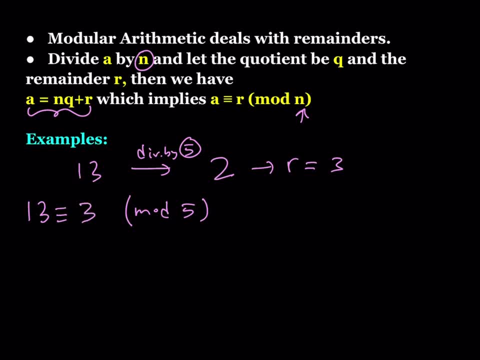 3, mod 5.. That's how you can basically write it. Here the quotient doesn't really matter. What matters is the remainder, okay. So we're not necessarily saying that. you know, a is congruent to r. mod n implies that the 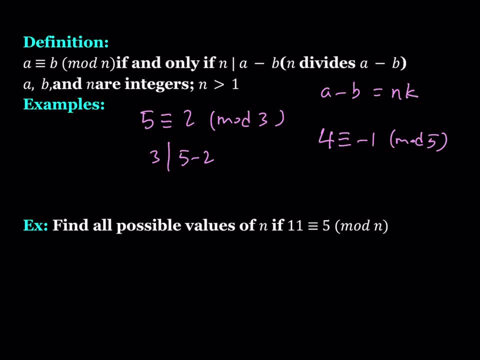 negative numbers as well. This is also true because, if you think about it, 5 divides 4 minus negative 1.. Here we have to be careful when subtracting a negative number. Okay, Let's take a look at this example here. This is one of the first examples that I actually 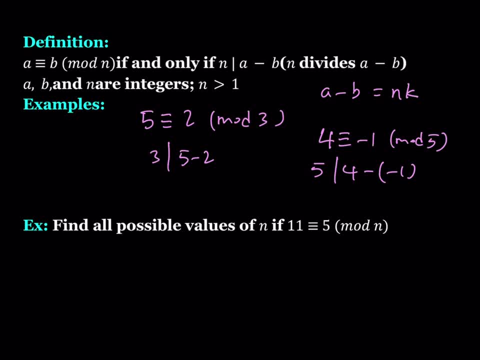 go over when I teach modul arithmetic: Find all possible values of n. if 11 is congruent to- so that's how we read it- congruent to 5 mod n. So in this case we don't know the modulus, We're trying to find it. and we do know that 11 is always congruent to 5.. 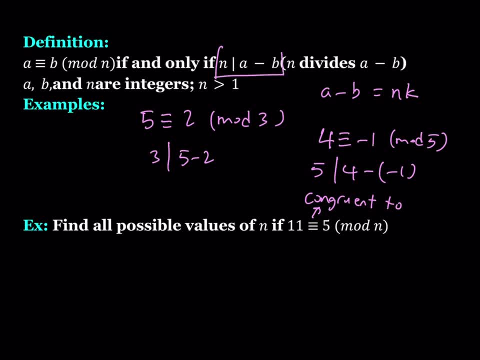 So we can use our formal definition. Basically what it means is: if a is congruent to 5, the to b mod n, then n divides a minus b. So we can safely say that n divides 11 minus 5, which means: 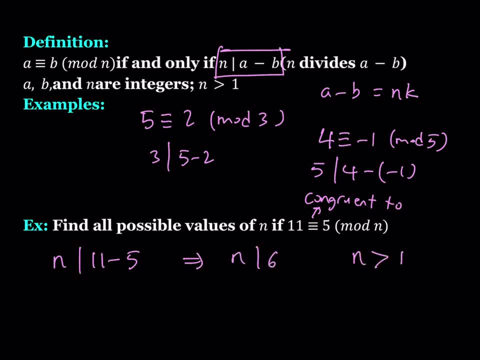 n divides 6.. And, of course, n needs to be greater than 1, and it's going to be an integer. So what integers divide 6?? We have 1,, 2,, 3, and 6.. Since we're not going to count 1,, we have 2,, 3, and 6.. 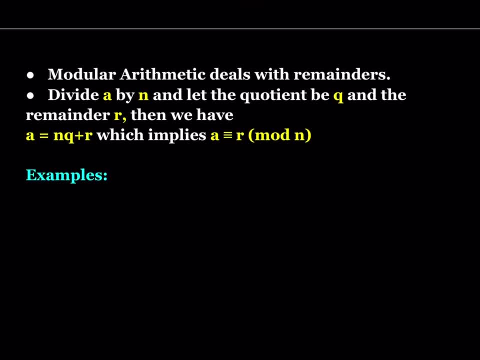 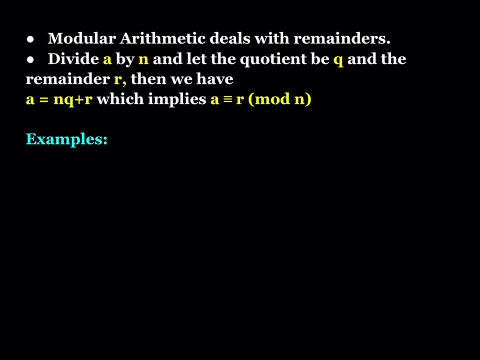 These are going to be the possible values of n. Okay, great. Now modular arithmetic. Why do we use modular arithmetic? It deals with remainders. So if you take a positive integer, a, and divide it by n, another positive integer, and let the quotient be q and the remainder r, then from 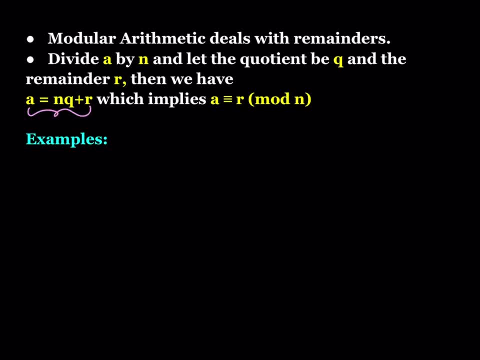 division algorithm. we can basically write the following, which implies: a is congruent to r mod n. Let me go ahead and explain this with an example. So suppose you're dividing 13 by 5, right? Well, of course, when you divide it by 5, the quotient is going to be 2,. 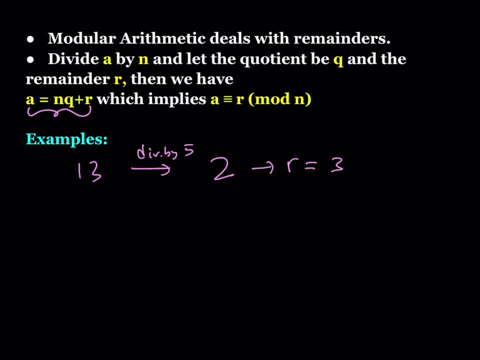 and the remainder is going to be 3, right, Okay. so what is that supposed to mean? It means that in this mod, which is mod 5, we're talking about mod 5 here because we're dividing by 5.. Remember, when you divide by n. 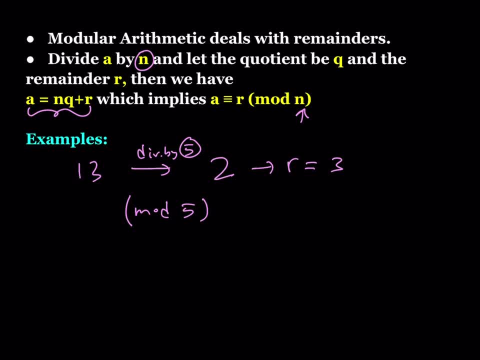 you're talking about mod n. Okay, so when we divide 13 by 5, we're getting a remainder of 3 mod 5.. That's how you can basically write it Here. the quotient doesn't really matter. What matters is the remainder. okay. 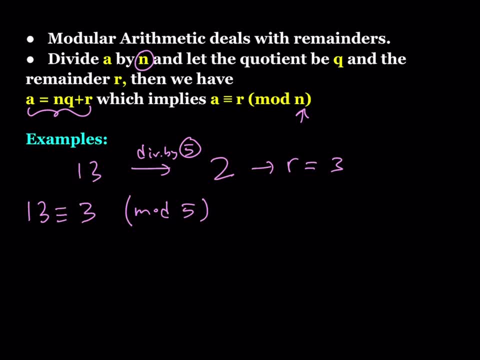 So we're not necessarily saying that. you know, a is congruent to r. mod n implies that the remainders are, but it's actually the other way around. Okay, we're going to be looking at more examples, So let me just go ahead and move forward, So we don't spend too much time on this. 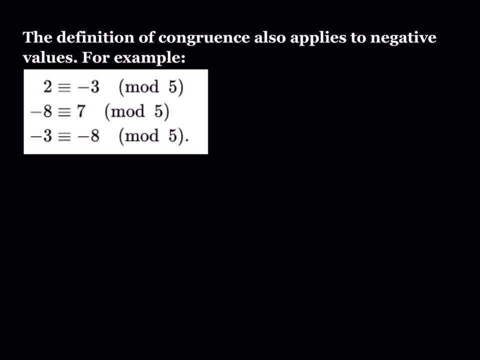 topic. The definition of congruence also applies to negative values, Like we talked about before. 2 is congruent to negative 3 mod 5, negative 8 is congruent to 7, and negative 3 is congruent to negative 8.. All these statements are true And you can always check. 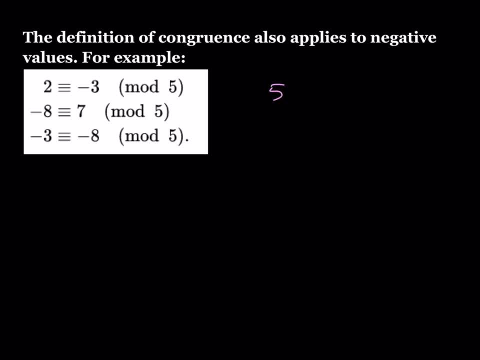 by looking at, for example. the first one is going to be: 5 divides 2 minus negative 3,, which is true. 5 divides negative 8 minus 7,, which is again true. And 5 divides negative 3 minus. 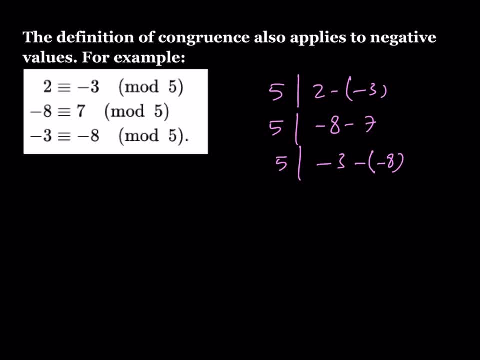 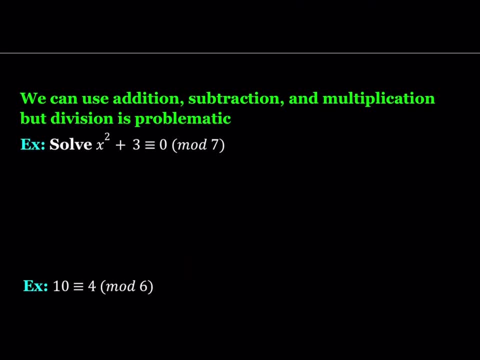 negative 8.. All right, all of these are true statements. So that's how you can basically use negative values, And they're very helpful sometimes. I'll show you a couple examples where they are extremely helpful. For example, this one: we can use addition. Okay, so one of the 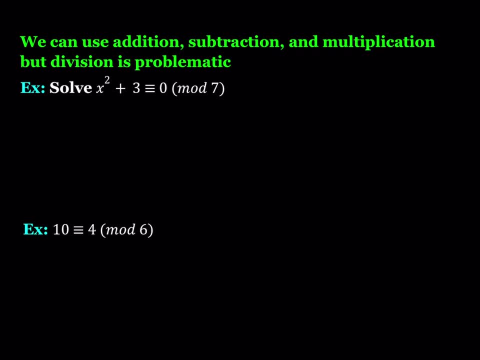 things that you can do, since it's a system of arithmetic. but you're doing it with a finite number of integers, which is kind of cool. you're allowed to do pretty much the same thing that you do normally, So you can add the same. 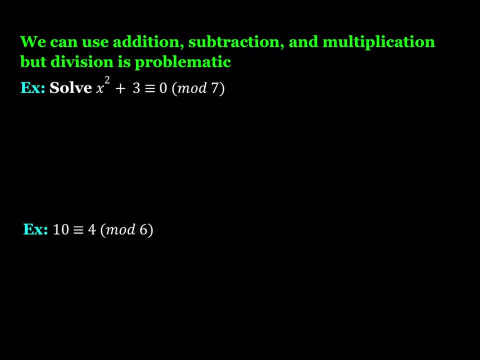 number. you can subtract the same number, you can multiply by the same number. but division is kind of problematic. We're going to look at division in the next example. So let's solve this equation. for example, Since I can subtract 3 from both sides, this gives me x. squared is congruent to. 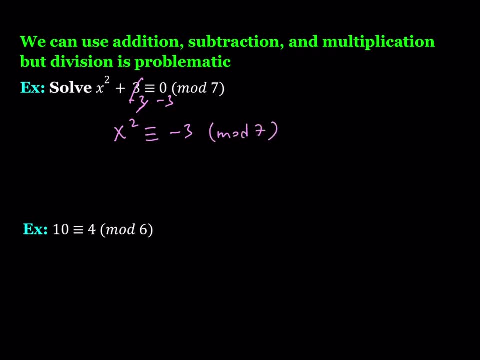 negative 3 mod 7.. Now, obviously negative 3 as a perfect square doesn't make sense and we're not going to go into the i business here. you know we're going to keep it real, for reals. Okay, so x squared is congruent to negative 3 mod 7.. How can I handle this? Well, 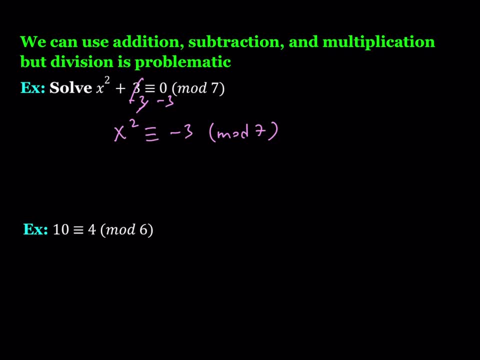 I can add 7 to both sides, because one of the things that we should always keep in mind is 7 is congruent to 0 mod 7.. Why? Because the difference between 7 and 0 is divisible by 7.. 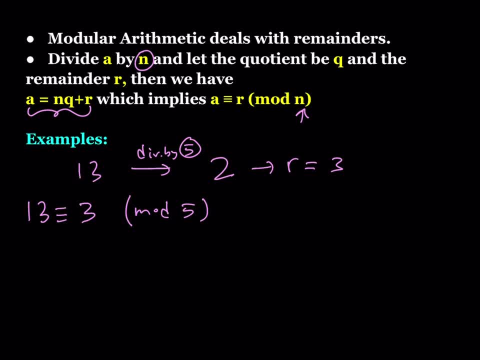 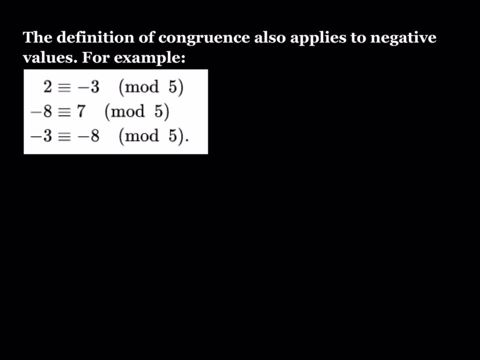 remainders are, but it's actually the other way around. Okay, we're going to be looking at more examples, So let me just go ahead and move forward, So we don't spend too much time on this topic. The definition of congruence also applies to negative values, Like we talked about before. 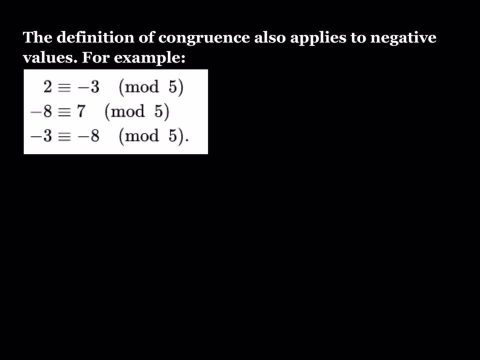 2 is congruent to negative 3 mod 5, negative 8 is congruent to 7, and negative 3 is congruent to negative 8.. All these statements are true And you can always check by looking at, for example. the first one is going to be 5 divides 2 minus negative 3,. 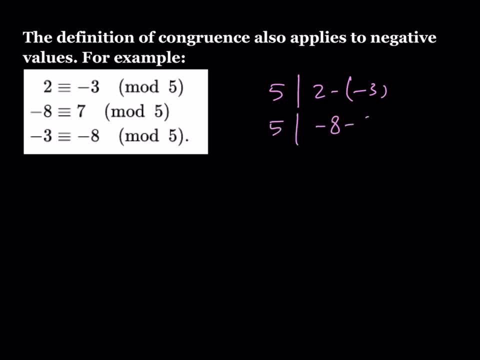 which is true. 5 divides negative 8 minus 7, which is again true. And 5 divides negative 3 minus negative 8.. All right, all of these are true statements, So that's how you can basically use negative values, And they're very helpful sometimes. I'll show you a couple examples where 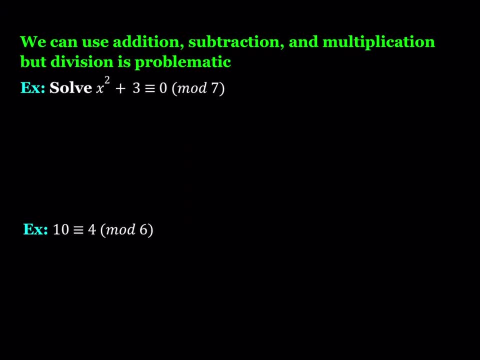 they are extremely helpful, For example, this one. we can use addition. Okay, so one of the things that you can do, since it's a system of arithmetic, but you're doing it with a finite number of integers, which is kind of cool. 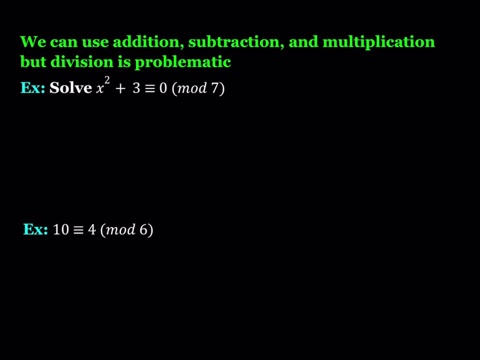 you're allowed to do pretty much the same thing that you do normally, So you can add the same number, you can subtract the same number, you can multiply by the same number. but division is kind of problematic. We're going to look at division in the next example, So let's solve this equation. 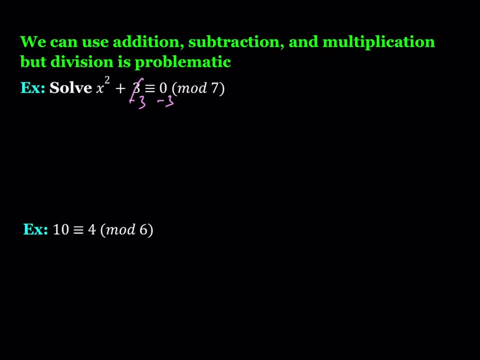 for example, Since I can subtract 3 from both sides, this gives me x squared is congruent to negative 3 mod 7.. Now, obviously negative 3 as a perfect square doesn't make sense and we're not going to go into the i business here. you know. we're going to keep it real. 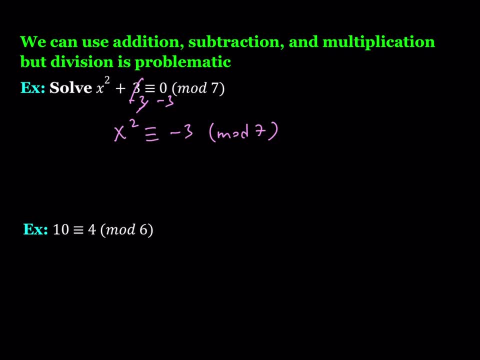 for reals. Okay, so x squared is congruent to negative 3, mod 7.. How can I handle this? Well, I can add 7 to both sides, because one of the things that we should always keep in mind is 7. 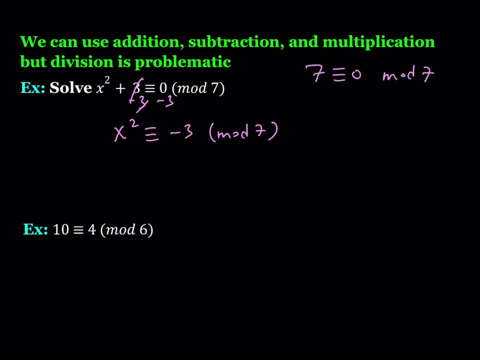 is congruent to 0 mod 7. Why? Because the difference between 7 and 0 is divisible by 7. So this is always true. So we can safely say that n is congruent to 0 mod n all the time, which is. 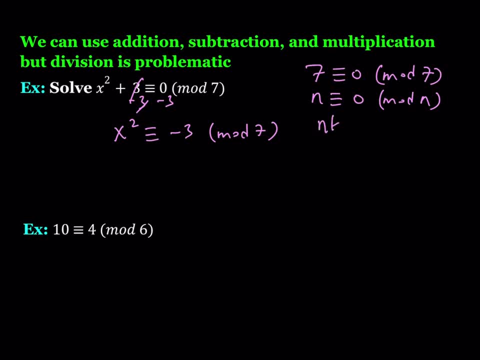 really good to know, And we can generalize this even more. like nk, if you have a multiple of n, it's always going to be 0 mod n as well. So this is good to know. Now I can just go ahead and add. 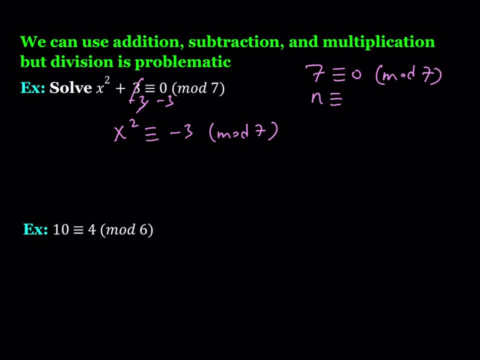 So this is always true. So we can safely say that n is congruent to 0 mod n all the time, which is really good to know. And we can generalize this even more: like nk, if you have a multiple of n, it's always going to be 0 mod n as well. So this is good to know. Now I can just go ahead and add: 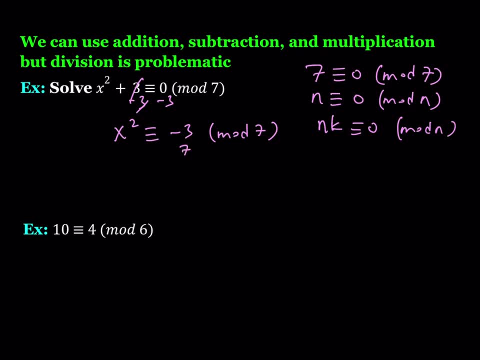 7 to both sides. But remember that 7 is congruent to 0.. So instead of adding 7 here, I can just add 0 on the left hand side. So this gives me x squared is congruent to 4 mod 7.. Now this is nice. 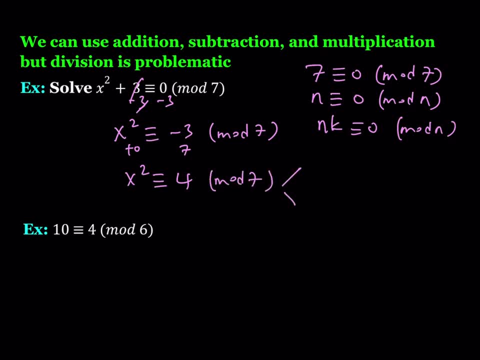 because 4 is a perfect square And from here I kind of branch off and say x is either 2, congruent to of course, or negative 2 mod 7.. But remember, we're allowed to add 7 or multiples of. 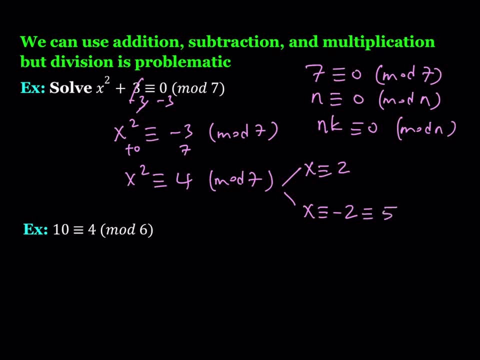 7.. So negative 2 is congruent to 5 mod 7.. So in mod 7, this equation has two solutions: 2 and 5.. And when I say mod 7, you should always think about this finite set: 0,, 1,, 2,, 3,, 4,, 5, and 6,. 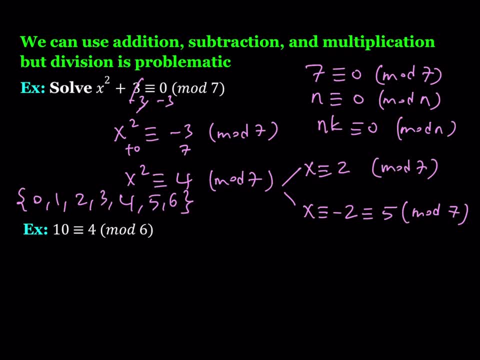 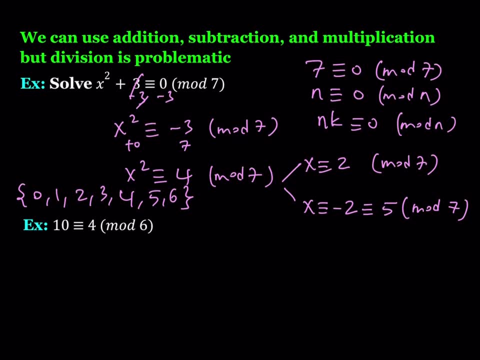 because these are the all possible remainders upon division by 7.. That's pretty much what we're dealing with. Now, if you look at the second example here on this page, we said that division is problematic. Let's illustrate why that's the case. If you divide, for example, well, 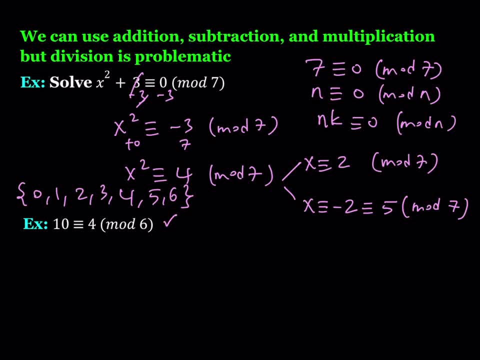 is this true? First of all, let's go ahead and check that: Is 10 congruent to 4 mod 6?? Yes, because 10 minus 4 is 6.. You see, there's a quick way to check that. You don't even have to go to. 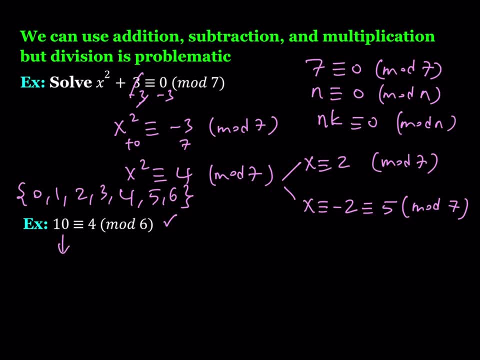 remainder business here, But anyways. so let's go ahead and divide both sides by 2, because 2 is a common factor. So is it true that 5 is congruent to 2 mod 6? Well, obviously that's not true. 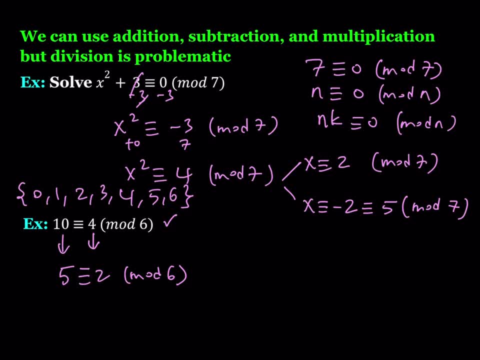 because if you think about 5 mod 6, it can be congruent to 5 mod 6 itself, or you can add 5 and write it as 11, or subtract 6 and write it as negative 1.. So we're not going to have 2 being 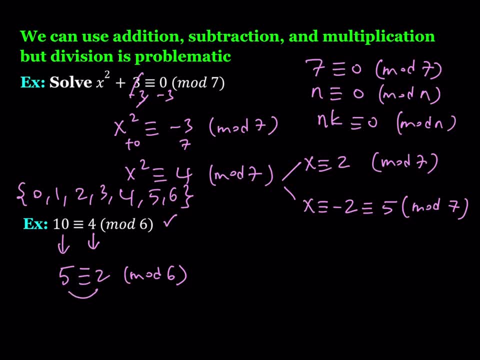 congruent to 5.. And you can also obviously check that 5 minus 2 is equal to 3, and 6 obviously does not divide 3.. Or I should probably write it more clearly as 5 minus 2, so it makes more sense. 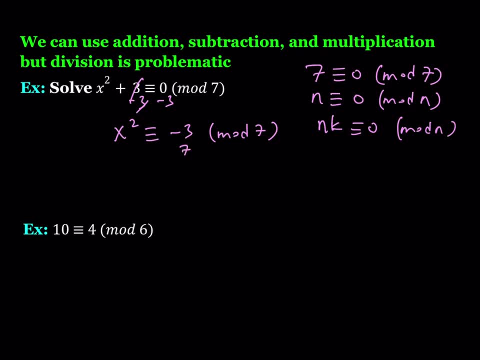 7 to both sides. But remember that 7 is congruent to 0.. So instead of adding 7 here, I can just add 0 on the left hand side. So this gives me x squared is congruent to 4 mod 7.. Now this is nice. 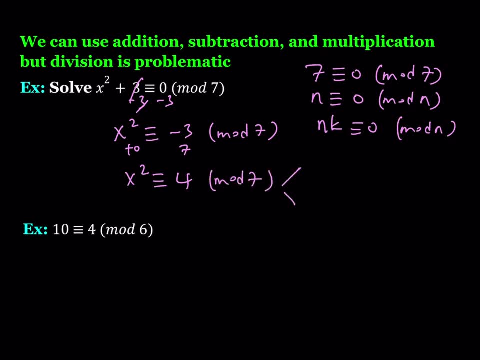 because 4 is a perfect square And from here I kind of branch off and say x is either 2, congruent to of course, or negative 2 mod 7.. But remember, we're allowed to add 7 or multiples. 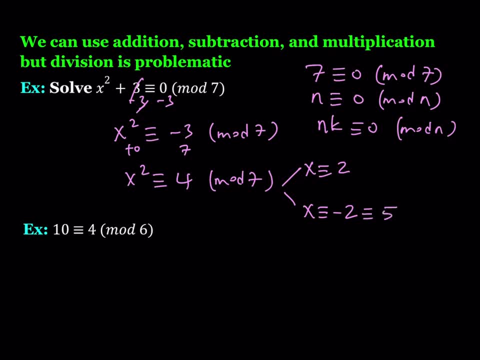 of 7.. So negative 2 is congruent to 5 mod 7.. So in mod 7, this equation has two solutions: 2 and 5.. And when I say mod 7, you should always think about this finite set: 0,, 1,, 2,, 3,, 4,, 5, and 6,. 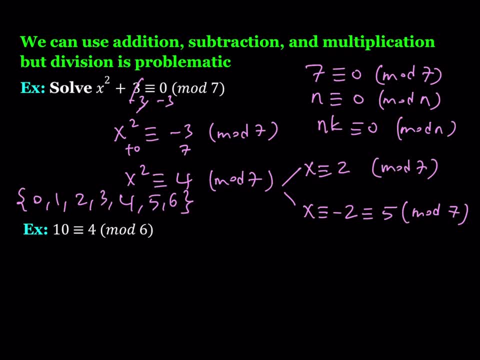 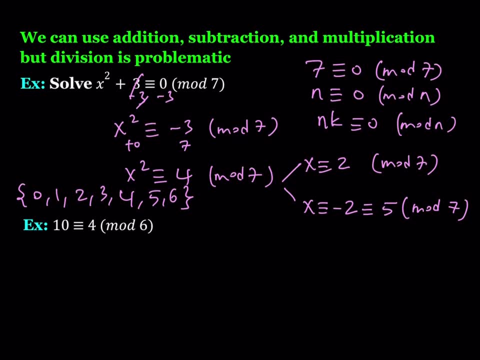 because these are the all possible remainders upon division by 7.. That's pretty much what we're dealing with. Now, if you look at the second example here on this page, we said that division is problematic. Let's illustrate why that's the case. If you divide, for example, well, 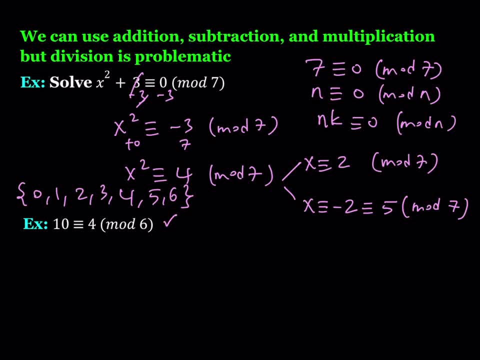 is this true? First of all, let's go ahead and check that: Is 10 congruent to 4 mod 6?? Yes, because 10 minus 4 is 6.. You see, there's a quick way to check that. You don't even have to go to. 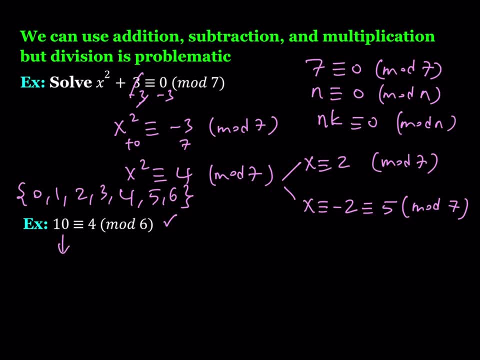 remainder business here, But anyways. so let's go ahead and divide both sides by 2, because 2 is a common factor. So is it true that 5 is congruent to 2 mod 6?? Well, obviously that's not true. 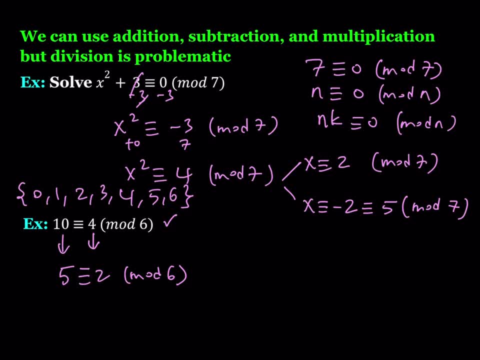 because if you think about 5 mod 6, it can be congruent to 5 mod 6 itself, or you can add 5 and write it as 11, or subtract 6 and write it as negative 1.. So we're not going to have 2 being 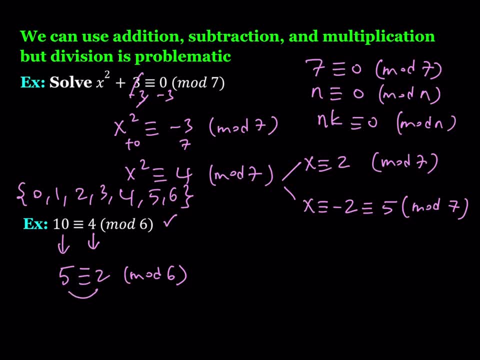 congruent to 5.. And you can also obviously check that 5 minus 2 is equal to 3, and 6 obviously does not divide 3.. Or I should probably write it more clearly as 5 minus 2, so it makes more sense. 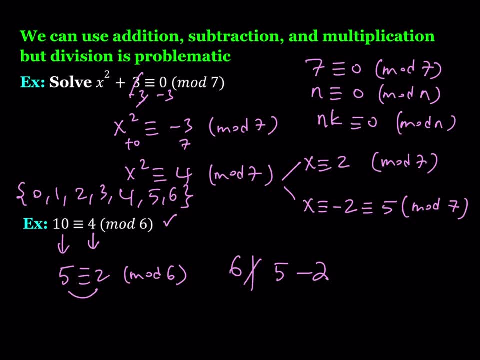 right. Okay. so division is problematic and there is a way to overcome that. sometimes, because we have a common divisor, If you divide both sides, including the mod, by 2, then you'll be good to go. Okay, let's take a look at this example. This is kind of interesting. 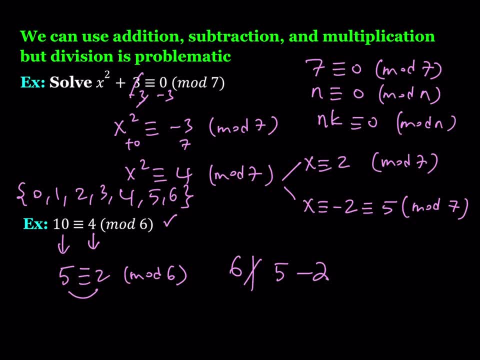 right. Okay. so division is problematic and there is a way to overcome that. sometimes, because we have a common divisor, If you divide both sides, including the mod, by 2, then you'll be good to go. Okay, let's take a look at this example. This is kind of interesting. 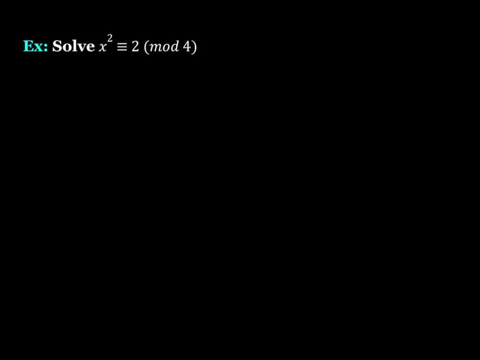 and this kind of puts us in a position where one of our additional topics talks about quadratic residues and stuff like that. So this is a really fun topic, but we'll talk about that later. Anyways, what number in mod 4 squared is going to be congruent to 2? When you think about 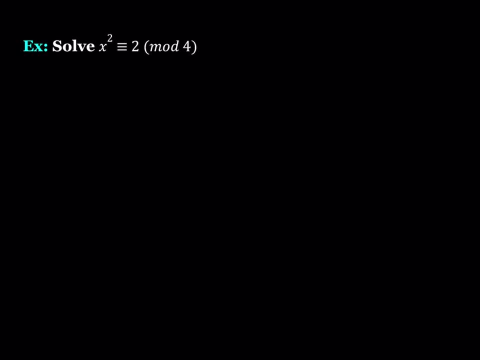 this. you might be thinking: okay, I'm going to add 4 to both sides, You can make the 6, you can make like 10, so on and so forth, but you'll never get a perfect square. Well, 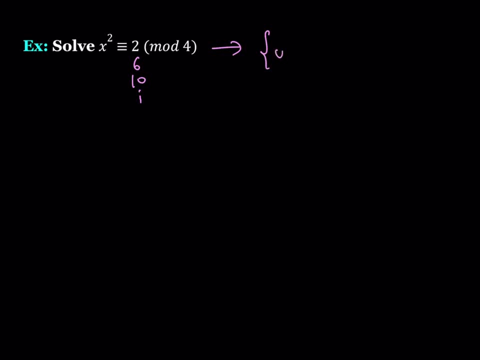 let's see what happens. When I say mod 4, you should understand this list right: 0,, 1,, 2,, 3.. So these are possible remainders, These are possible numbers in mod 4.. So let's go ahead. 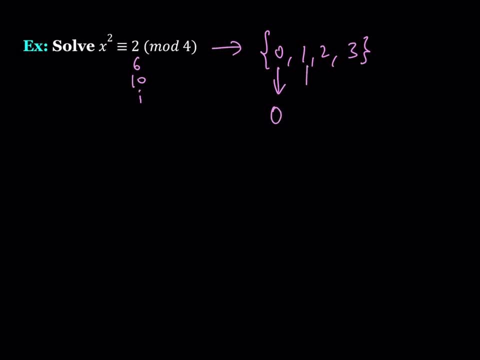 and square each one of them. For example, 0 squared is 0 mod 4,, 1 squared is 1 mod 4, 2 squared is 4 mod 4, but let's go ahead and write it as 0, and 3 squared is 9,. but if you divide it, 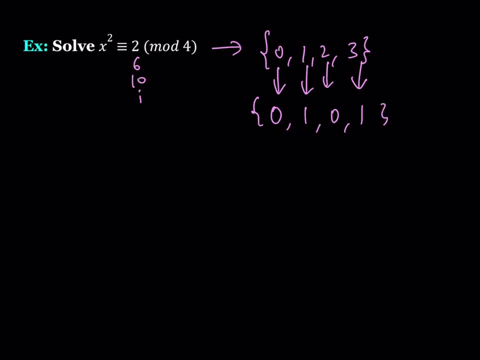 by 1 mod 4.. So all these numbers, so this is the set of Xs and this is the set of X squares, right? What do you notice? Well, if you square a number and you look at it, mod 4, it's never going to. 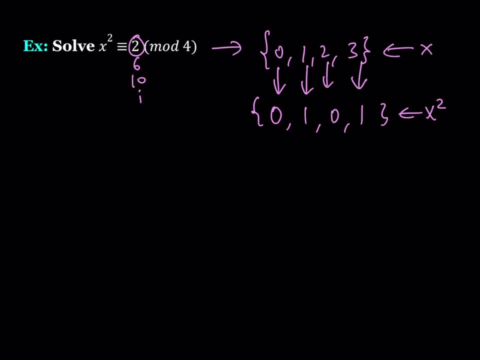 equal or it's never going to be congruent to 2 mod 4.. So this equation has no solution, because a perfect square can never be 2 mod 4.. And you can easily verify this. Think about well, this basically means that X is even, And if you square it, you can easily verify this. So you can easily. 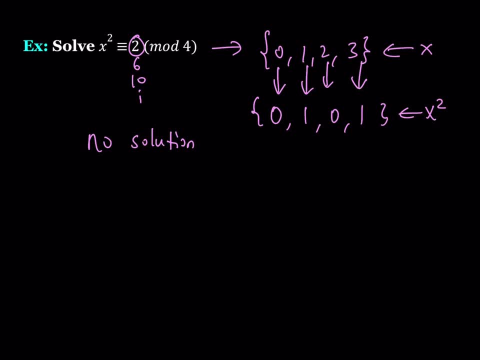 square even numbers, you're going to notice that they're never going to leave a remainder of 2. Mod 4. Okay, Cool, So this equation has no solution. What about negative exponents? Well, we're talking about negative exponents, but there are no negative exponents. Well, 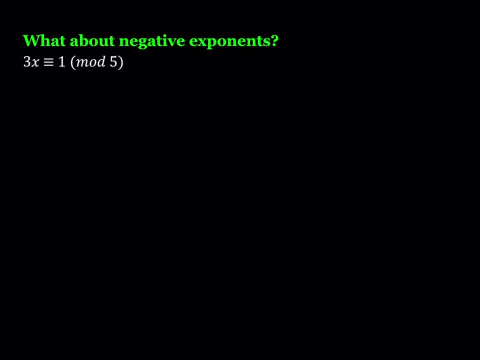 here's what we're going to do. We're going to go with. first of all, let me tell you, division is not like a standard procedure, So we don't really write like one-third. One-third, like a fraction, is not defined in mod 5 or in any mod. So what we're going to do instead is: 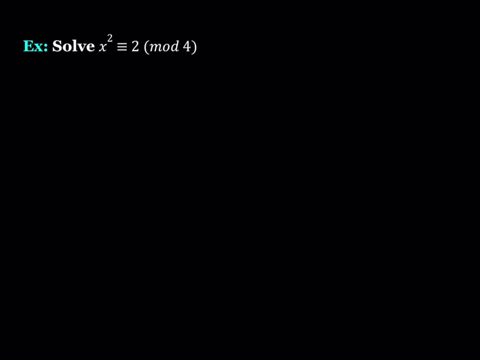 and this kind of puts us in a position where one of our additional topics talks about quadratic residues and stuff like that. So this is a really fun topic, but we'll talk about that later. Anyways, what number in mod 4 squared is going to be congruent to 2? When you think about 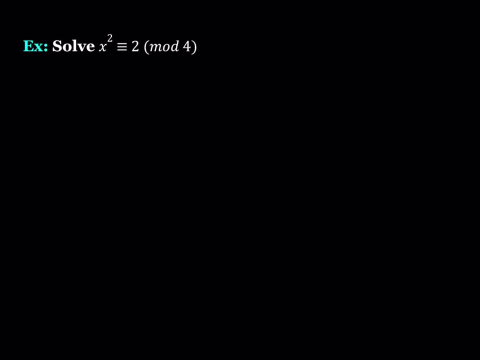 this, you might be thinking: okay, I'm going to add 4 to both sides, You can make this 6, you can make like 10, so on and so forth, but you'll never get a perfect square. Well, let's see what happens. When I say mod 4, you should understand this list right? 0,. 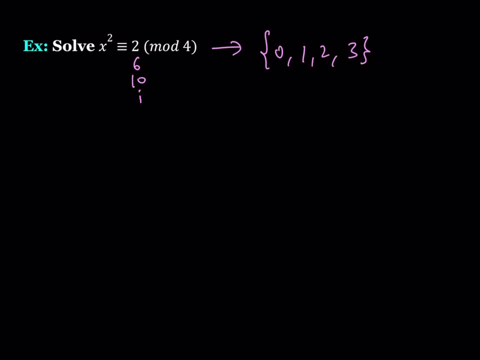 1,, 2, 3.. So these are possible remainders, These are possible numbers in mod 4.. So let's go ahead and square each one of them. For example, 0 squared is 0 mod 4, 1 squared is 1 mod 4,. 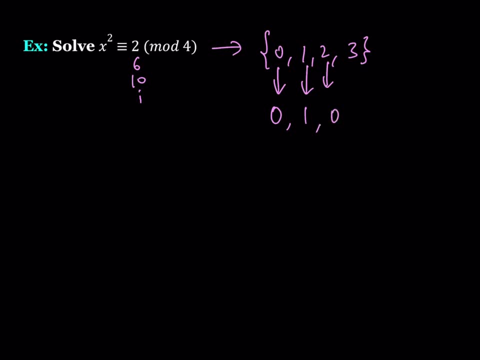 2 squared is 4 mod 4, but let's go ahead and write it as 0, and 3 squared is 9, but if you divide it by 4 and look at the remainder, you're going to get get 1 mod 4.. So all these numbers, so this is the set of x's and this is the set of x. 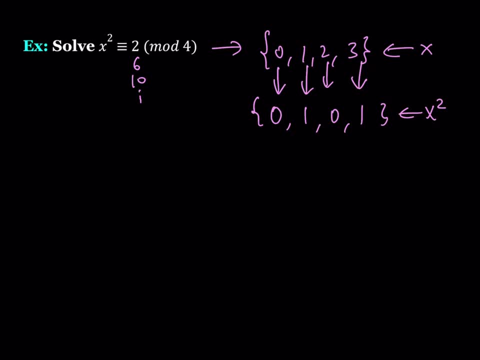 squares right. What do you notice? Well, if you square a number and you look at it, mod 4, it's never going to equal or it's never going to be congruent to 2 mod 4.. So this equation has no solution, because a perfect square can never be 2 mod 4.. And you can easily. 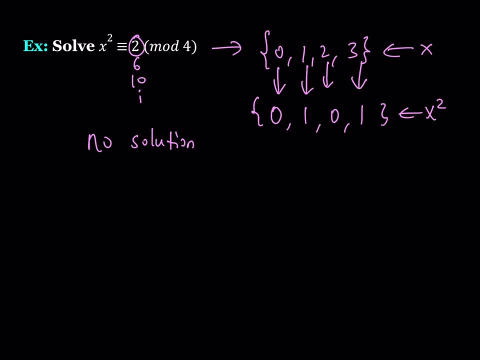 verify this. Think about, well, this basically means that x is even, And if you square even numbers, you're going to notice that they're never going to leave a remainder of 2 mod 4.. Okay, cool, So this equation has no solution. What about negative exponents? Well, we're. 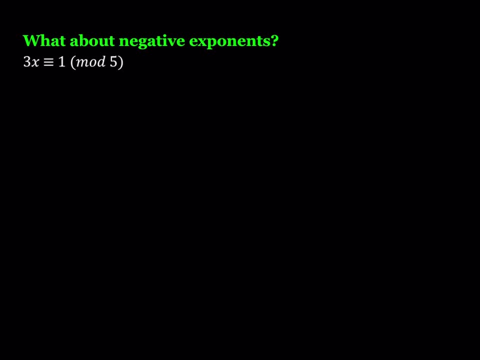 talking about negative exponents, but there are no negative exponents. Well, here's what we're going to do. We're going to go with. first of all, let me tell you, division is not like a standard procedure, So we don't really write like one third, One third, like. 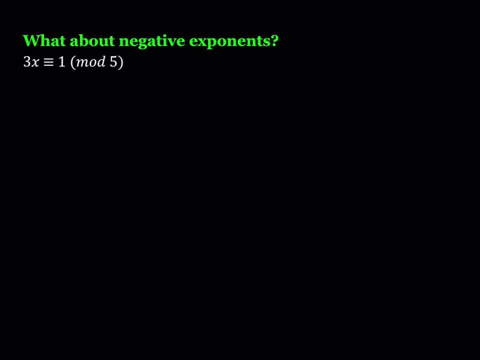 a fraction is not defined in mod 5. Or in any mod. So what we're going to do instead is multiply both sides by the inverse of 3.. So let's go ahead and multiply both sides by 3 inverse And let's see what happens. 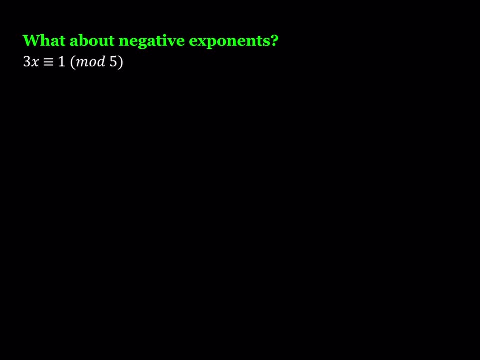 multiply both sides by the inverse of 3.. So let's go ahead and multiply both sides by 3 inverse and let's see what happens. Of course I'm multiplying from the left to be kind of like exact. That's what we're going to get. So this gives you. now, when you multiply a number by 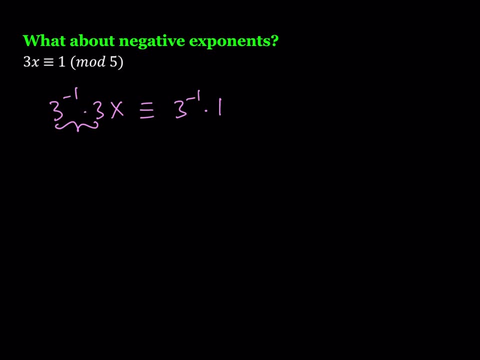 its inverse. obviously, that's going to give you the identity element which, when multiplied by x, gives you x. So this is basically going to be like a 1 in multiplication. So we're going to be getting x from here, and when you multiply by 1, of course it's going to be the same symbol. 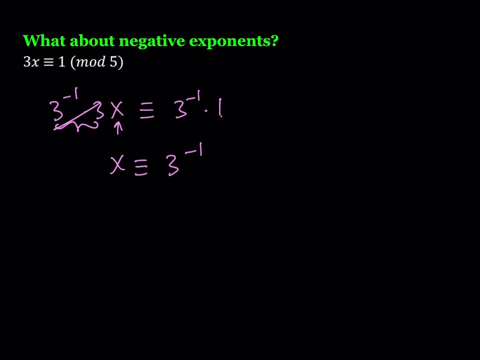 In other words, the number we're looking for is the inverse of 3 mod 5.. But how do you find the inverse of a number, or any number, to the negative exponent? Well, let's go ahead and think about this: Mod 5,. 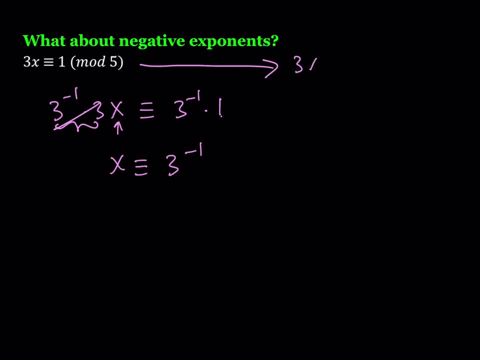 I'm allowed to add 5 or multiples of 5.. So let's go ahead and add 5 to 1 to make it 6. And this equation is definitely solvable. You can divide both sides by 3, because 3,, 6, and 5 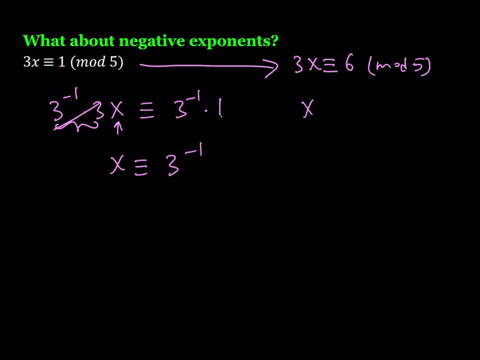 do not have a common factor. So we can go ahead and divide and that's going to give us x is congruent to 2 mod 5. And that's basically going to be the solution. So the inverse of 3 is 2 mod 5, which means the 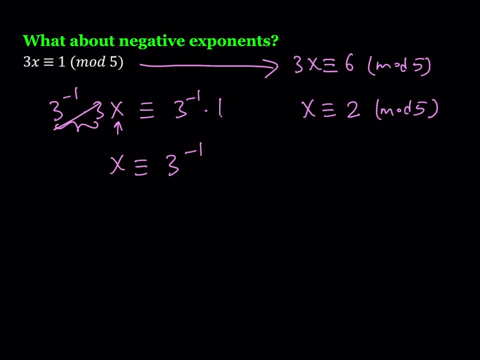 inverse of 2 is also 3.. So 2 and 3 are inverses, mod 5.. In any mod can we find inverses. That's not always the case, because you can't always get a 1.. All right, that's another interesting topic. 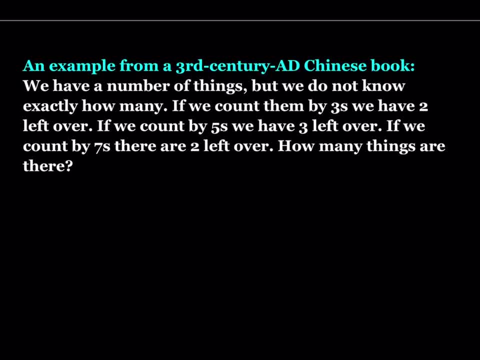 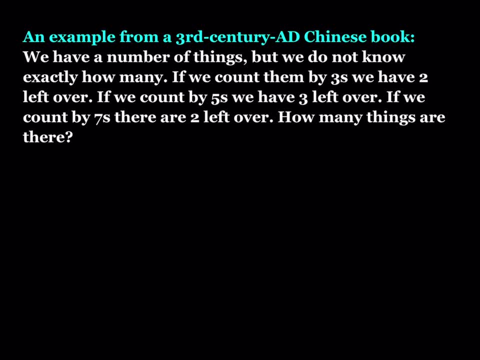 which I'm going to leave open-ended for now. Now let's take a look at this example. This is an example from a 3rd century AD Chinese book. You've probably seen similar problems. These are fairly common. We have a number of things, but we do not know how many. We count them. 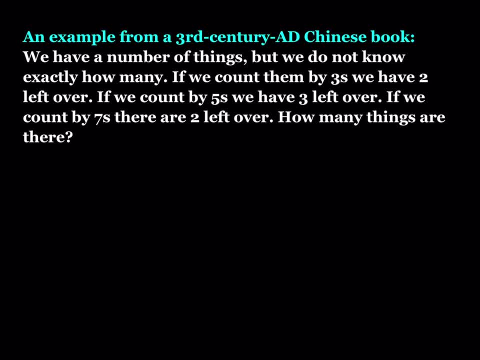 by 3s, we get. we have 2 left over. If you count by 5s, 3 left over and 7s, we have 2 left over. So we can actually write this as a system of congruences. How Well the number we're looking. 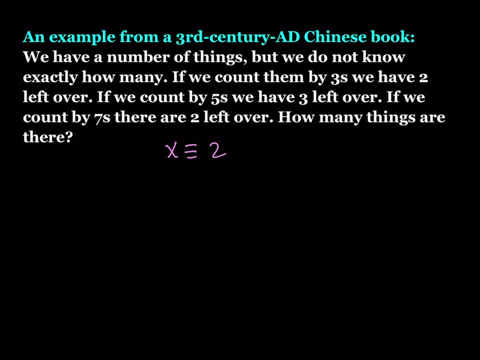 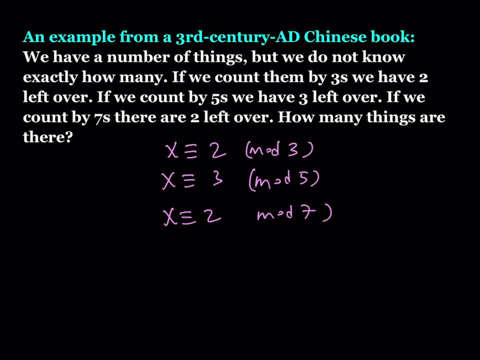 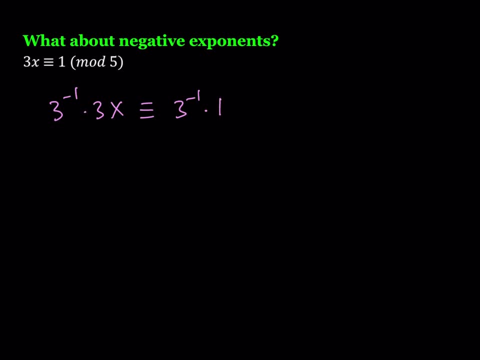 Of course I'm multiplying from the left, to be kind of like exact. That's what we're going to get. So this gives you. now, when you multiply a number by its inverse, obviously that's going to give you the identity element which, when multiplied by x, gives you x. So this 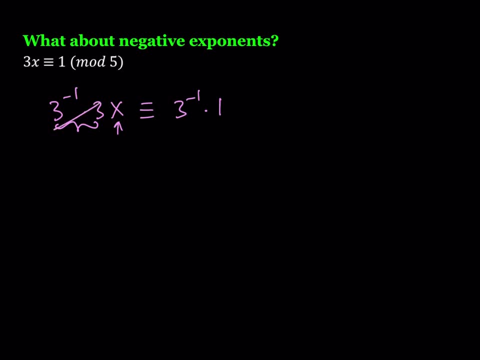 is basically going to be like a one in multiplication. So we're going to be getting x from here, And when you multiply by one, of course it's going to give you x. So what we're going to do is we're going to multiply x by 1.. And we're going to multiply x by 1.. So this is going to 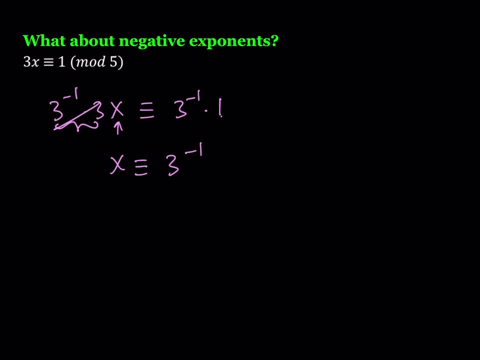 it's going to be the same symbol. In other words, the number we're looking for is the inverse of 3 mod 5.. But how do you find the inverse of a number, or any number, to the negative exponent? Well, let's go ahead and think about this. Mod 5, I'm allowed to add 5 or multiples of 5.. So let's go. 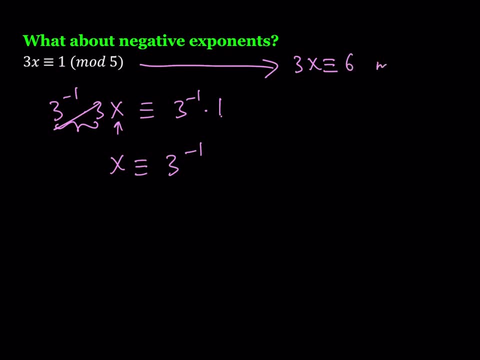 ahead and add 5 to 1 to make it 6.. And this equation is definitely solvable. You can divide both sides by 3, because 3,, 6, and 5 do not have a common factor. So we can go ahead and divide. 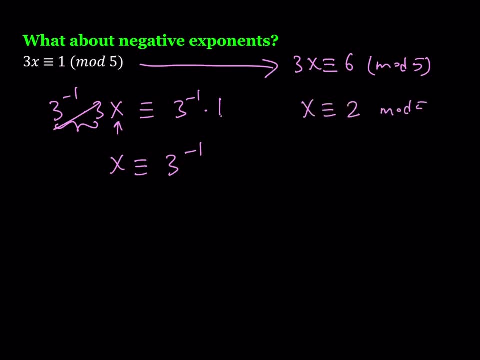 and that's going to give us x is congruent to 2 mod 5. And that's basically going to be the solution. So the inverse of 3 is 2 mod 5, which means the inverse of 2 is also 3.. So 2 and 3. 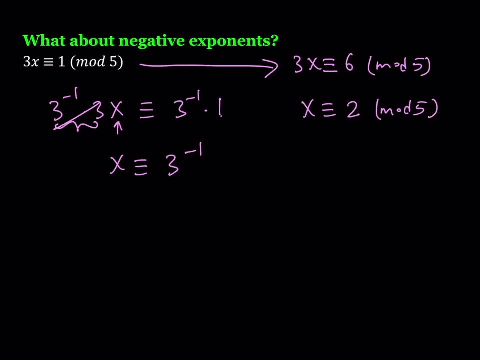 are inverses, mod 5. In any mod can we find inverses. That's not always the case, because you can't always get a 1.. All right, that's another interesting topic which I'm going to leave open-ended for now. Now let's take a look at this example. This is an example from a third 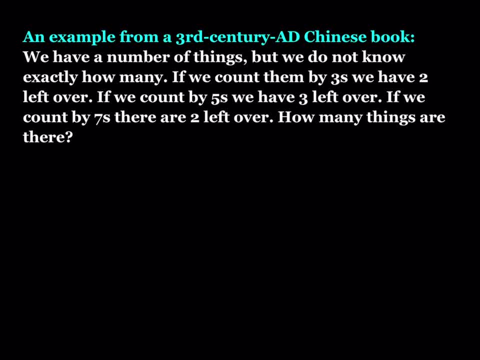 century AD Chinese book. You've probably seen similar problems. These are fairly common. We have a number of things, but we do not know how many. We count them by 3s, We have 2 left over. If you count by 5s, 3 left over And 7s, we have 2 left over. So we can actually write this as a system. 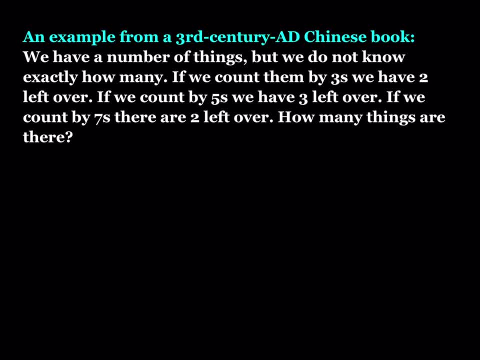 of congruences. How Well, the number we're looking for. let's call that x. x is going to be 2 mod 5.. I mean 2 mod 3.. x is congruent to 3 mod 5.. 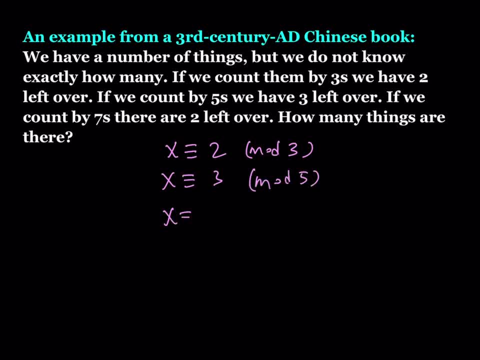 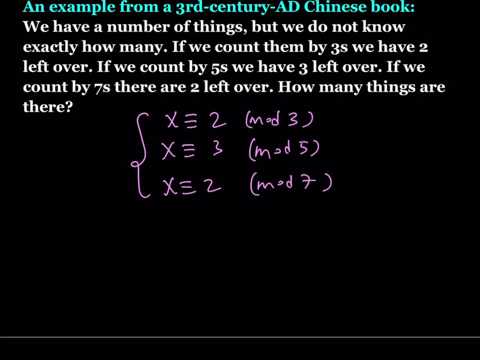 And x is congruent to 2 mod 7.. Obviously, this is a system of congruences And this system has a solution, And that solution in this case would be 23.. For example, if you think about the number 23, you're basically talking about something. when you divide by 3,, you're going to get a remainder. 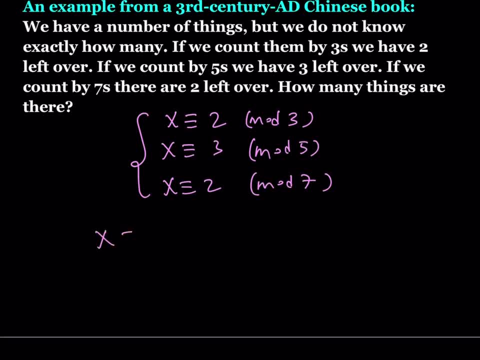 and this system has a solution, And that solution in this case would be 23.. For example, if you think about the number 23,. you're basically talking about something: when you divide by 3,, you're going to get a remainder of 2.. When you divide by 5, it's going to be 3.. And when you 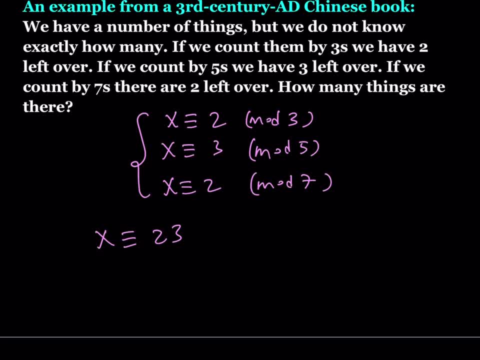 divide by 7, you're going to get 2. So x is congruent to 23.. So 23 satisfies the system. But to be able to find this and solve this- of course with higher mods it's much harder- 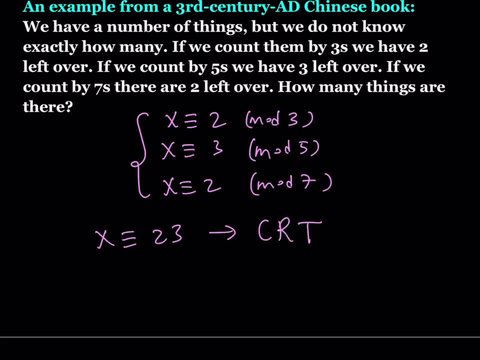 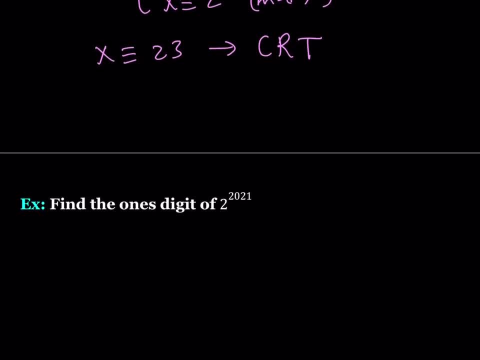 We have something called Chinese remainder theorem, which I also included in additional topics. Okay, That's a very interesting topic, something that we're probably going to talk about later. So modular arithmetic deals with remainders, we said, And of course it also deals with 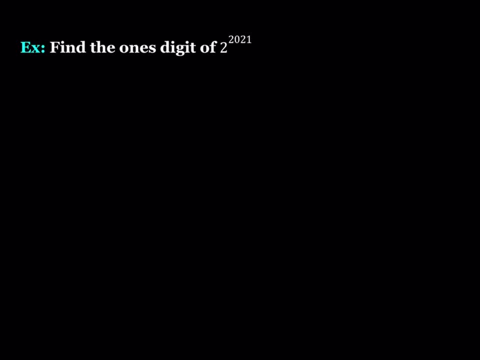 problems like this. For example, we use modular arithmetic to find the ones digit of this number. Obviously, this is a very large number, right, You would probably agree. Like just to give you an idea about the magnitude, just an approximate. 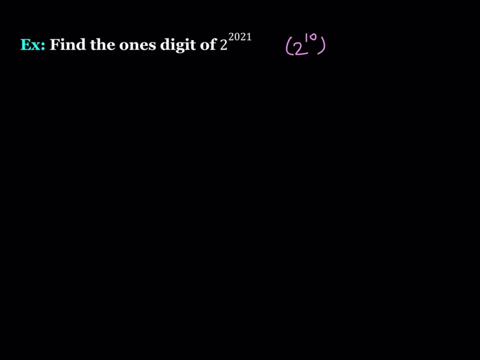 Like 2 to the 10th power is pretty close to, you know, 1,000, which is 10 to the 3rd power. So if you raise 2 to the 10th power, so I can probably safely say that something like: 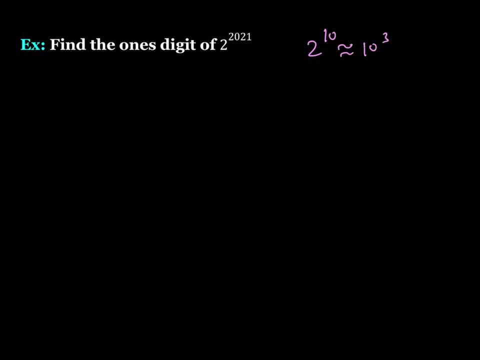 2 to the 10th is close to 10 to the 3rd, And then if I raise this to the power 200, that's going to be close to well, kind of 10 to the power, 3 to the power 200, which is like: 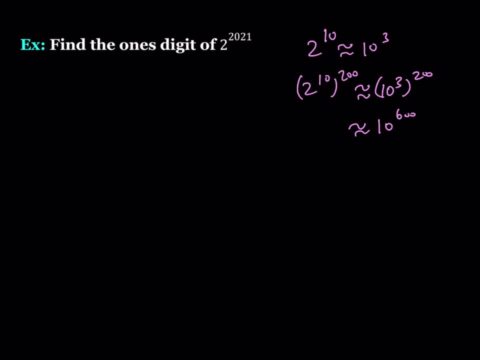 10 to the power 600. So you're basically talking about something one followed by, or at least something that's close to the power 200. So you're basically talking about something that has 600-something digits. right, That's a really large number, Obviously. 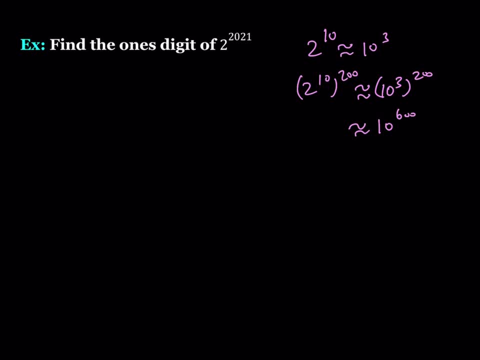 we're not going to calculate that and we're not even going to look at the ones digit of this number. Obviously, there's an easier way to do it. When they say ones digit, you would always think about it. if I divide a number by 10, the remainder is going to be the ones digit, right? 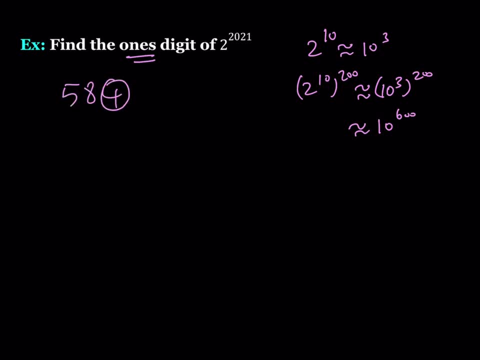 So if you have 584, the remainder is 4, obviously, Or if you have 100, the remainder will be 0. So what we need to do, then, is work in mod 10.. How do you work in mod 10?? 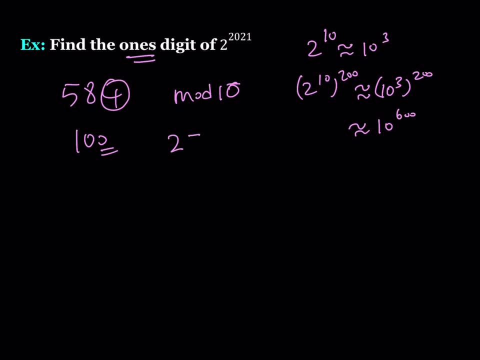 And we're going to be evaluating this number. So let me go ahead and do the following: 2 is 2 mod 10.. So what I'd like to do is I'd like to raise 2 to higher power. So this is 2 to the. 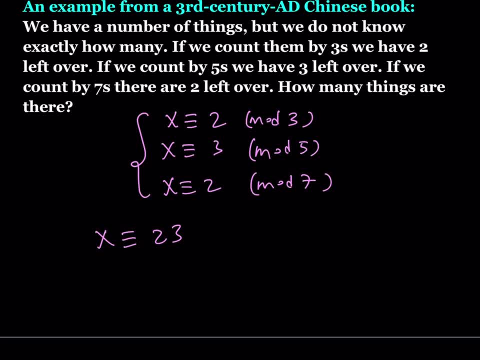 of 2.. When you divide by 5, it's going to be 3.. And when you divide by 7, you're going to get 2.. So x is congruent to 23.. So 23 satisfies the system. But to be able, 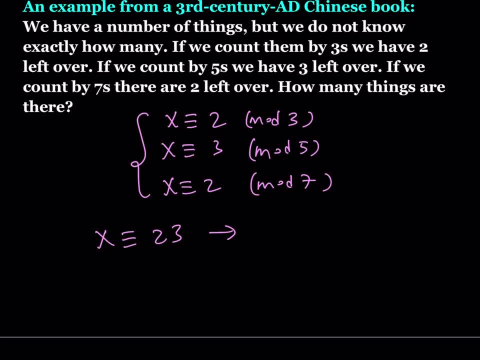 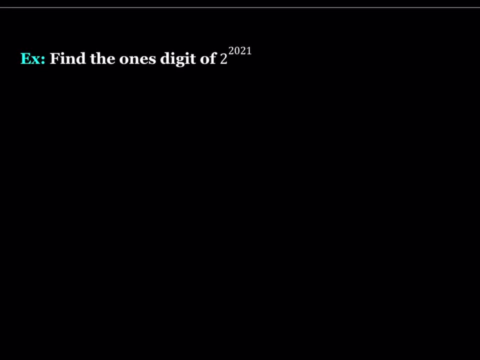 to find this and solve this. of course, with higher mods it's much harder. We have something called Chinese remainder theorem, which I also included in additional topics. Okay, That's a very interesting topic, Something that we're probably going to talk about later. So modular: 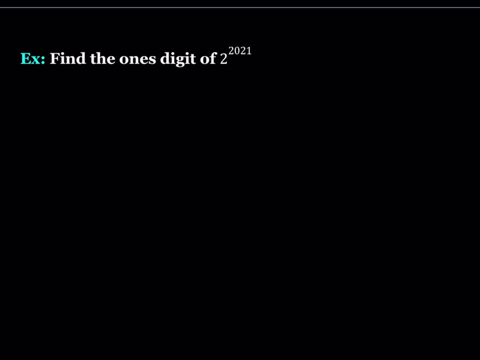 arithmetic deals with remainders, we said, And of course it also deals with problems like this. For example, we use modular arithmetic to find the ones digit of this number. Obviously, this is a very large number, right? You would probably? 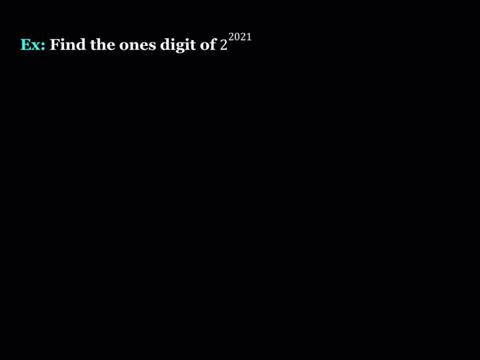 agree. Just to give you an idea about the magnitude, just an approximation like 2 to the 10th power is pretty close to 1,000, which is 10 to the third power. So if you raise 2 to the 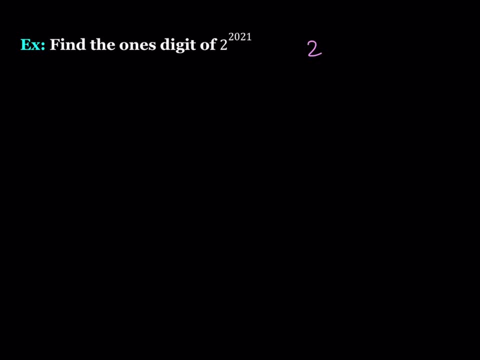 10th power. so I can probably safely say that something like 2 to the 10th is close to 10 to the third, And then if I raise this to the power 200, that's going to be close to well, kind of. 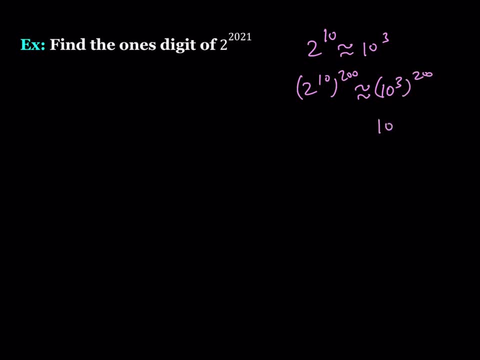 10 to the power, 3 to the power 200, which is like 10 to the power 600.. So you're basically talking about something, one followed by, or at least something that has 600 something digits. right, That's a really large number. Obviously, we're not going to calculate that and we're not. 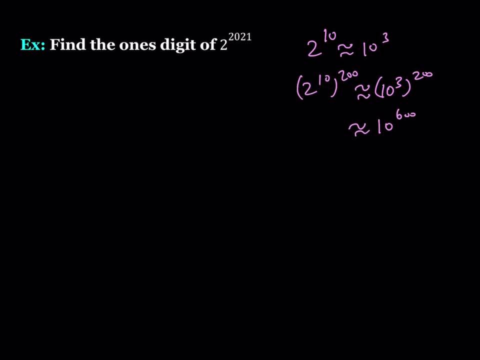 even going to look at the ones digit of this number. Obviously, there's an easier way to do it. When they say ones digit, you would always think about it. if I divide a number by 10, the remainder is going to be the ones digit, right? So if you have 584,? 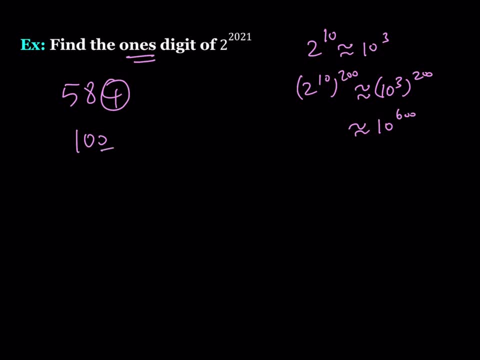 the remainder is 4, obviously. Or if you have 100, the remainder will be 0. So what we need to do, then, is to work in mod 10.. How do you work in mod 10?? We're going to be evaluating this number, So let 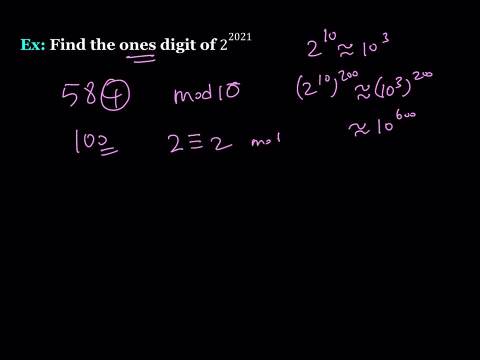 me go ahead and do the following: 2 is 2 mod 10.. So what I'd like to do is I'd like to raise 2 to higher power. So this is 2 to the first power. What about 2 to the second power? It's 4.. Again. 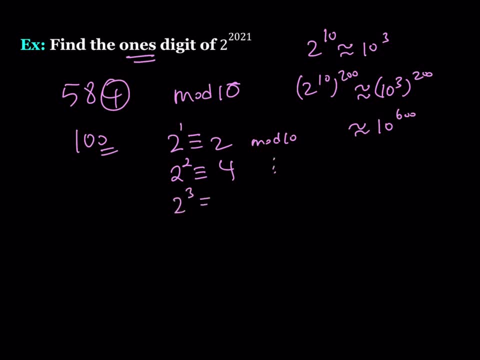 mod 10,. I'm not going to repeat it, but you know it's mod 10.. 2 to the third is 8, and then 2 to the fourth is 16, but I can write it as 6 because 6 and 16 are congruent mod 10.. So if you could, 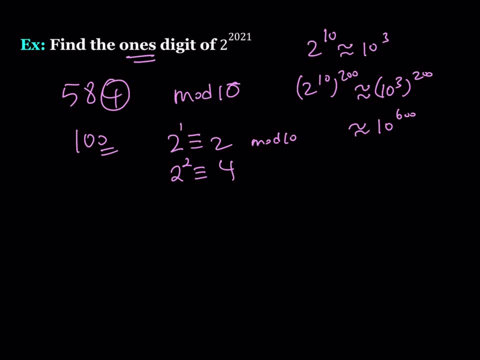 first power. What about 2 to the second power? It's 4.. Again, mod 10,. I'm not going to repeat it, but you know it's mod 10.. 2 to the third is 8, and then 2 to the fourth is 16, but I can write. 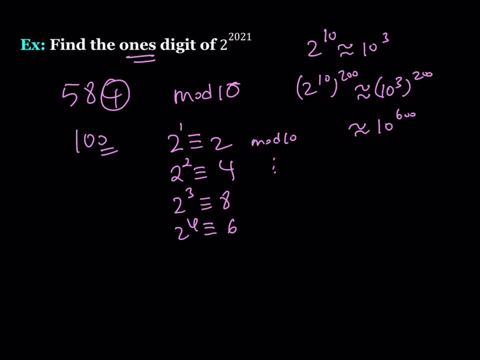 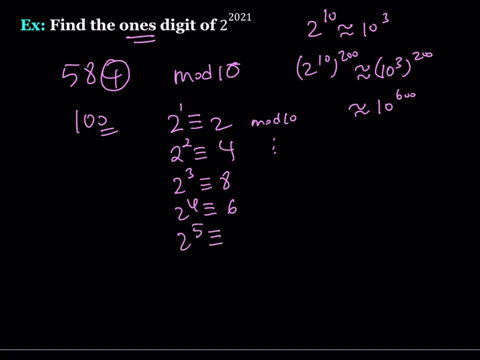 it as 6, because 6 and 16 are congruent mod 10.. So if you continue this pattern, you're going to notice that 2 to the fifth is 32.. Or just multiply the 6 by 2, you'll get 12,, which is 2 mod 10.. Now notice that this pattern 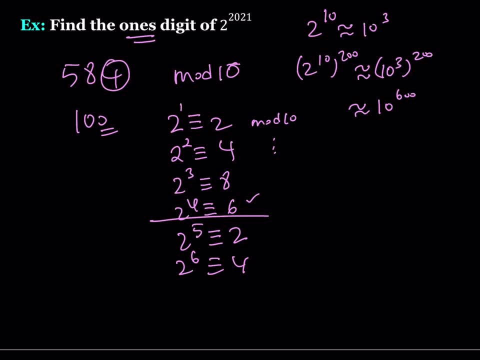 is going to start repeating, right, So it repeats. We have a cycle of 4.. Therefore, we just have to figure out where 2021 falls. And if you look at 1,, 2,, 3,, 4,, these are kind. 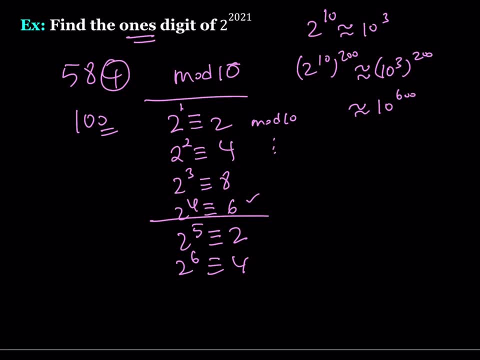 of like mod 4 numbers right? So 2021 is going to leave us a remainder of 1 when divided by 4.. So in other words, I can simply say that 2021 is 1 mod 4.. So it's going to be. 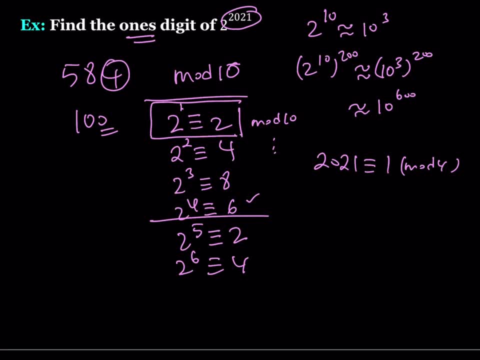 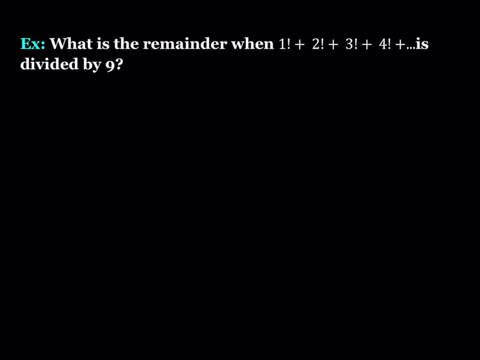 congruent to 1,, which means that the 1's digit is going to be 2.. Okay, Let's continue with more examples. What is the remainder when this number, the sum, infinite sum, is divided by 9?? So we have all these factorials and we're trying to divide by 9.. Now what? 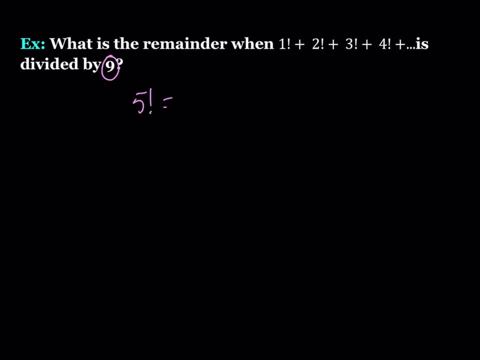 do you know about factorials? Well, 5 factorial is 120,, 6 factorial is 720, and this it's divisible by 720, right, I mean 9 divides 720,. in other words, Okay, Starting with 6 factorial. So here's what's going on. Let me go ahead and write more terms. 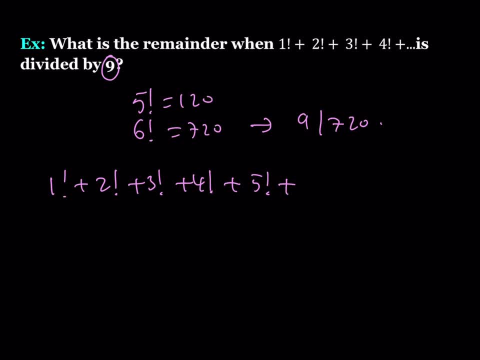 here to show you what's going on. Obviously, anything higher than 6 factorial contains 6 factorial. Therefore, all of these terms are divisible by 9.. Therefore, they leave a remainder of 0.. So the only thing that I need to look at is the first 5, and it's. 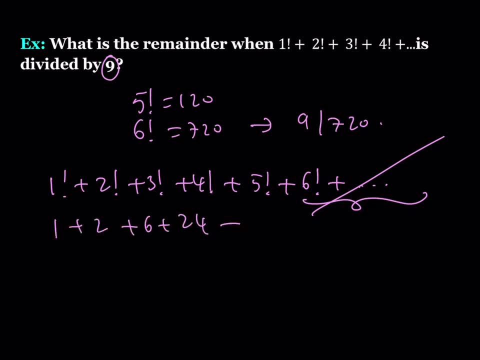 kind of like 1 plus 2 plus 6 plus 24 plus 120.. Obviously, this ends in 0.. Let's see what happens. This is going to give me a 30, 150, and that's going to be 150. 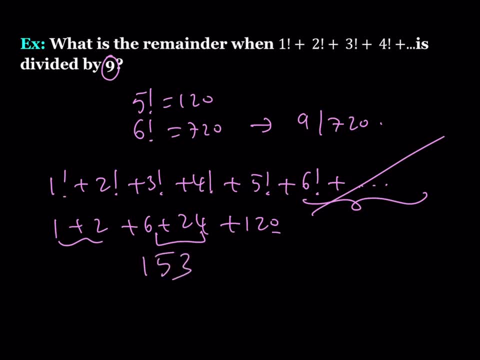 Now, how do you find the remainder when this number is divided by 9?? Well, you're just going to add up the digits and that's going to give you the answer. right, Okay, And that is 9.. Therefore, this number is going to be divisible by 9, which means it's going to 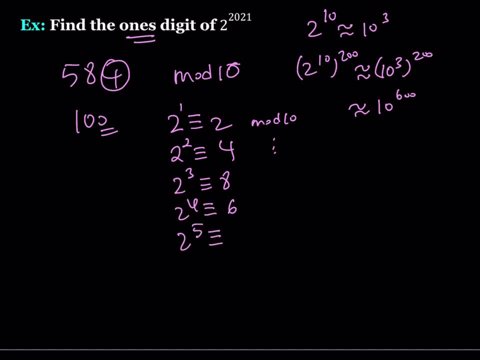 continue this pattern, you're going to notice that 2 to the fifth is 32, or just multiply the 6 by 2, you'll get 12,, which is 2 mod 10.. Now notice that this pattern is going to start repeating. 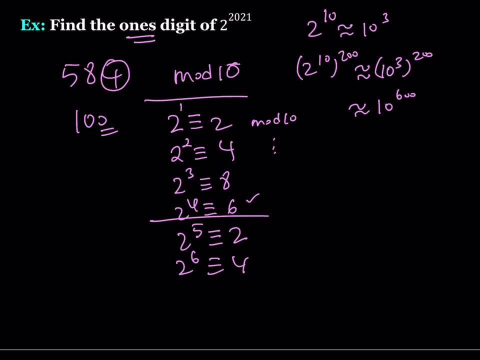 right? So it repeats: we have a cycle of 4.. Therefore, we just have to figure out where 2021 falls. And if you look at 1,, 2,, 3, 4, these are kind of like mod 4 numbers, right? So 2021 is. 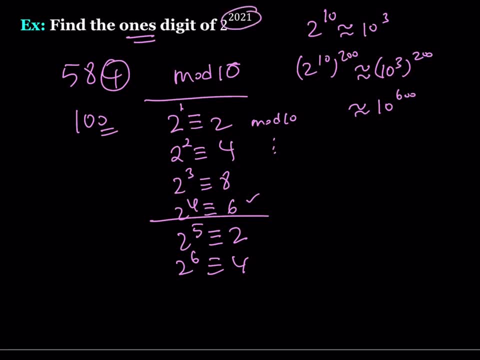 going to leave us a remainder of 1 when divided by 4.. So, in other words, I can simply say that 2021 is 1 mod 4.. So it's going to be congruent to 1,, which means that the 1's digit is going to be. 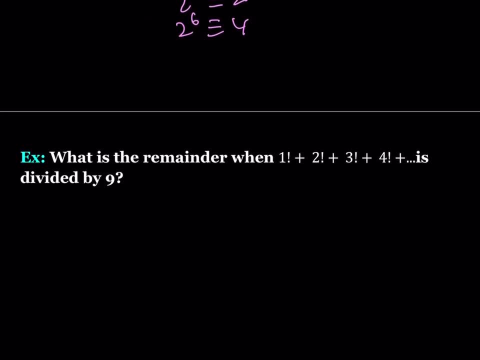 2.. Okay, let's continue with more examples. What is the remainder when this number, the sum, infinite sum, is divided by 9?? So we have all these factorials and we're trying to divide by 9.. Now, what do you know about factorials? Well, 5 factorial is 120,, 6 factorial is 720, and this 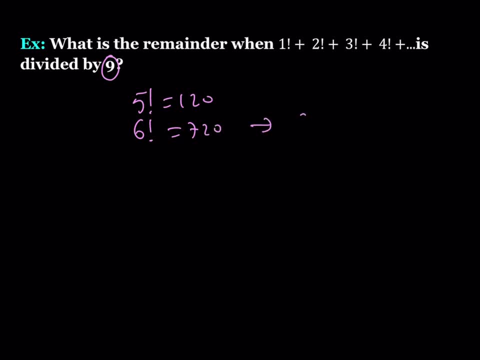 it's divisible by 720.. Right, I mean 9 divides 720, in other words, Okay. So starting with 6, factorial. so here's what's going on. Let me go ahead and write more terms here to show you what's going on, Obviously. 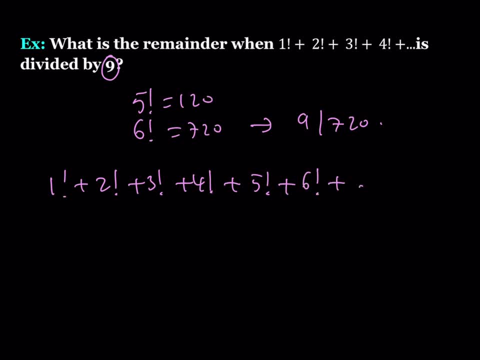 anything higher than 6 factorial contains 6 factorial. Therefore, all of these terms are divisible by 9.. Therefore, they leave a remainder of 0.. So the only thing that I need to look at is the first 5, and it's kind of like 1 plus 2 plus 6 plus 24 plus 120.. Obviously, this ends in 0.. 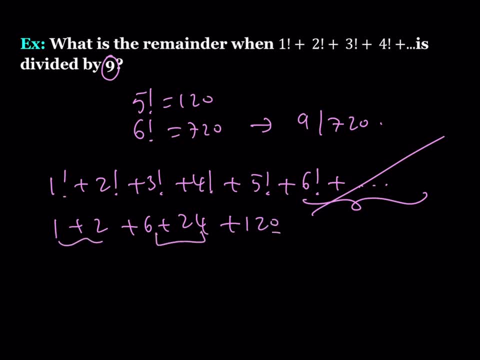 Let's see what happens. This is going to give me a 30,, 150, and that's going to be 153.. Now how do you find the remainder when this number is divided by 9?? Well, you're just going to add up the digits and that's going. 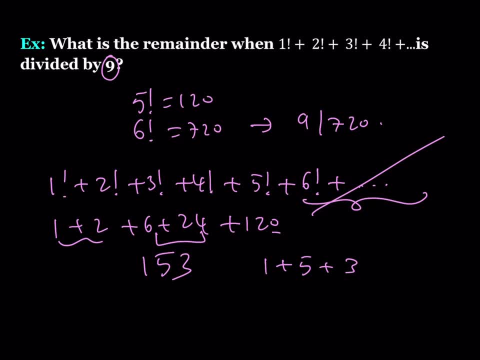 to give you the answer. Right, Okay, And that is 9.. Therefore, this number is going to be divisible by 9, which means it's going to leave the remainder of 0.. Okay, Cool, Let's take a look at another. 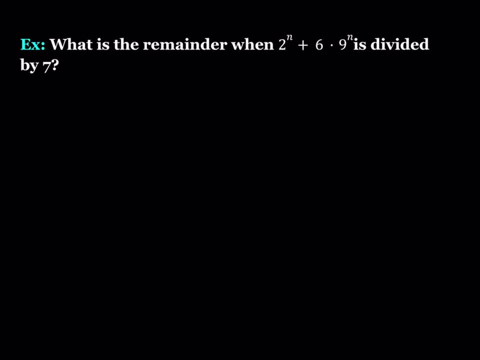 problem. What's the remainder? when 2 to the nth plus 6 times 9 to the nth, This is divided by 7.. Now here's one thing that you might be thinking. You might just plug in some values for n and see what's going on. right, I mean, that's probably going to work, because if 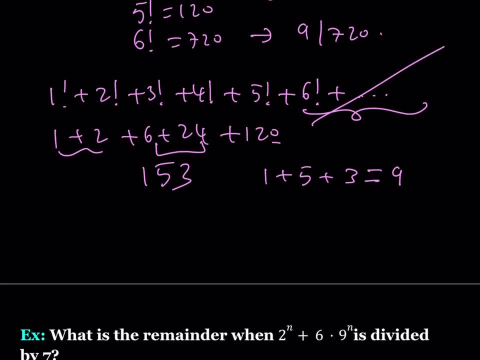 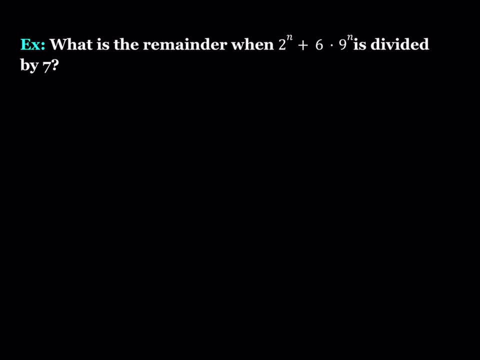 leave the remainder of 0.. Okay, Cool, Let's take a look at another problem. What's the remainder when 2 to the nth plus 6 times 9 to the nth is divided by 7? Now here's one thing. You might just plug in some values for n and see what's going on, right, I mean? 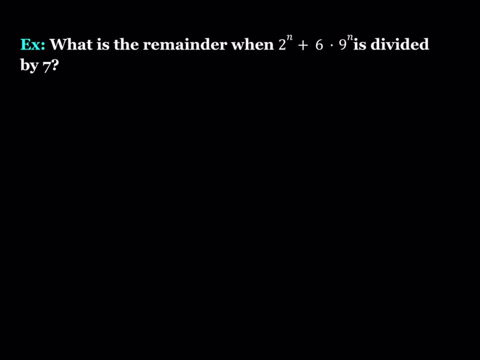 that's probably going to work, because if you have a fixed remainder, it should work with n equals 0, n equals 1, n equals 2, whatever. Well, in this case I guess we are defining n to be a positive integer. So let's say n is an element of positive integers, so that 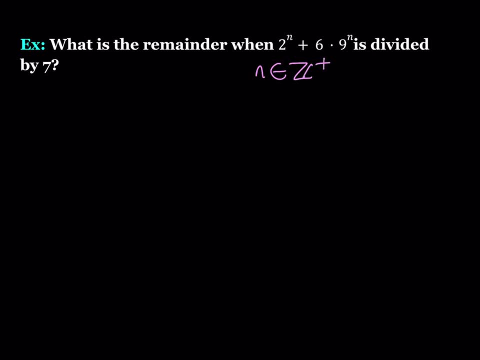 we don't have to deal with stuff like 0.. Okay, Now, how does this work? Here's what I can do: 9 to the nth, since 9 is congruent to 2 mod. 9 to the nth, since 9 is congruent to 2 mod. 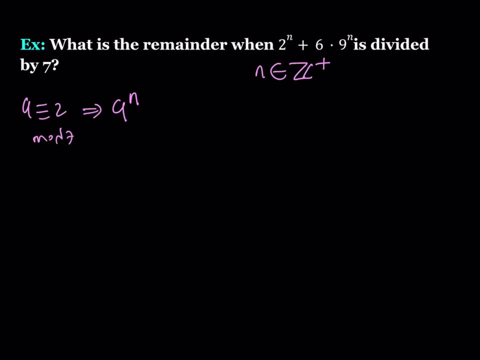 7, right, This is mod 7.. 9 to the nth is going to be congruent to 2 to the nth, because one of the things that I guess I forgot to say is: you can raise both sides to a power. You. 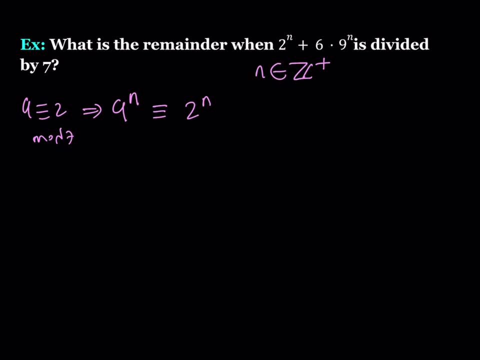 can add, multiply, subtract and raise both sides to a power, But division is a little tricky Now, so what I can do is I can basically replace this 9 to the nth with 2 to the nth, since they're congruent, And this gives me 1 times 2 to the nth plus 6 times 2 to the. 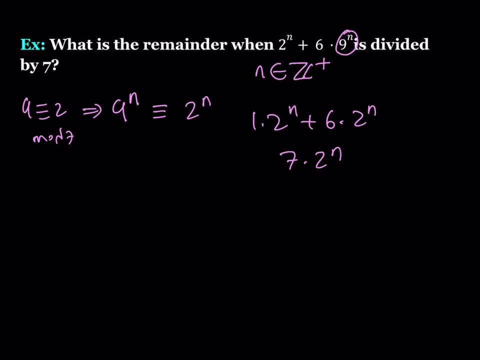 nth, which is 7 times 2 to the nth, And, as you know, any multiple of 7 is congruent to 0 mod 7.. Therefore, the remainder is again 0, when this number is divided by 7.. And you can again test it with certain values: All. 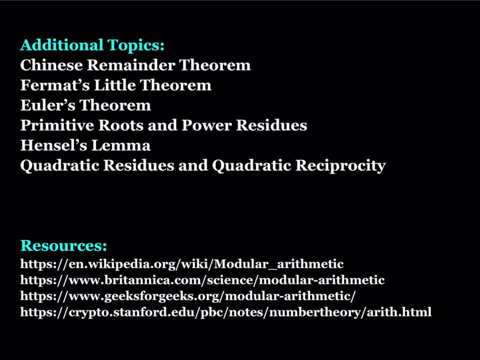 right, Cool Now. this brings us to the end of this video, but let me briefly talk about some additional topics here. Well, we have Chinese remainder theorem, which I briefly mentioned, to solve systems of congruences. Fermat's little theorem is very interesting. 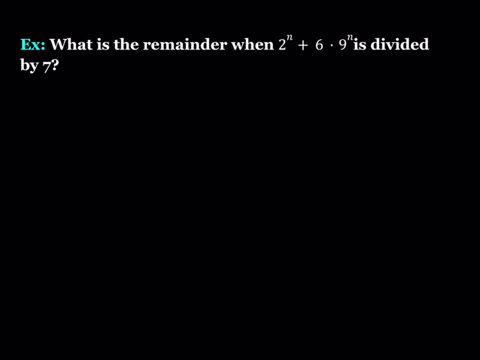 you have a fixed remainder. it should work with n equals 0, n equals 1, n equals 2, whatever. Well, in this case, I guess we are defining n to be a positive integer. So let's say n is an. 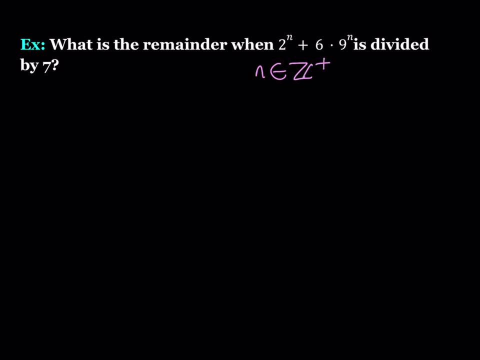 element of positive integers, so that we don't have to deal with stuff like 0.. Okay, Now how does this work? Here's what I can do: 9 to the nth, since 9 is congruent to 2 mod 7,. right, This is mod 7.. 9 to the nth is going to: 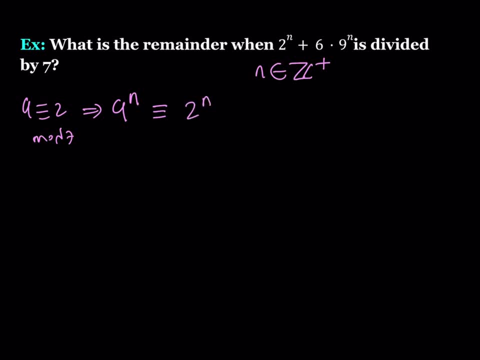 be congruent to 2 to the nth, because one of the things that I guess I forgot to say is you can raise both sides to a power. You can add, multiply, subtract and raise both sides to a power, But division is a little tricky Now, so what I can do is I can basically replace this 9 to the nth. 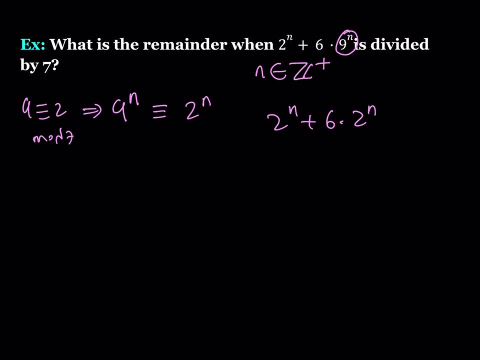 with 2 to the nth, since they're congruent, And this gives me one type of division. So I can add 2 to the nth. So what I've done is I can make a division with 6 to the nth, from 2 to the nth. 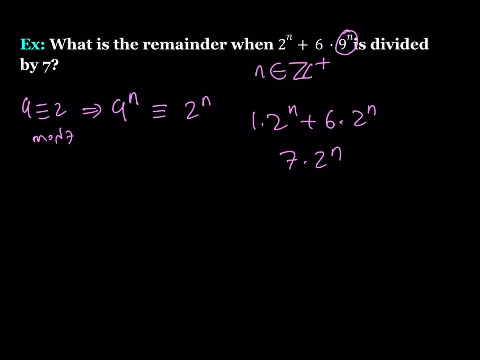 plus 6 to the nth, which is 7 to the nth, And, as you know, any multiple of 7 is congruent to 0 mod 7.. Therefore, the remainder is again 0 when this number is divided by 7.. And you can again test. 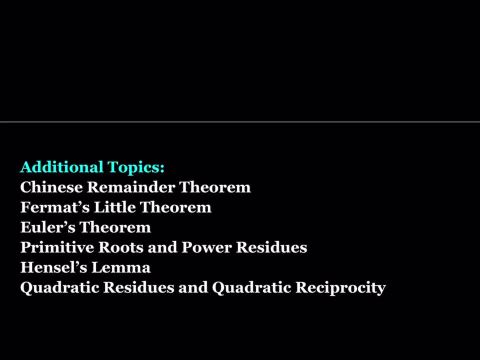 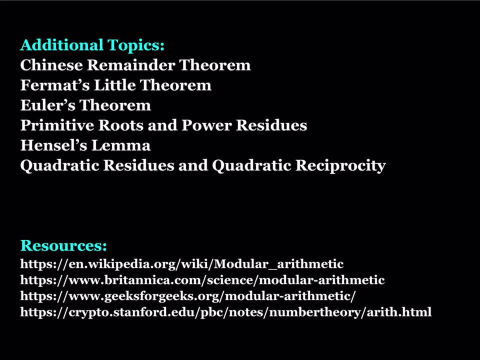 it with certain values. All right, Cool. Now, this brings us to the end of this video, but let me briefly talk about some additional topics here. Well, we have Chinese remainder theorem, which I briefly mentioned, to solve systems of congruences. 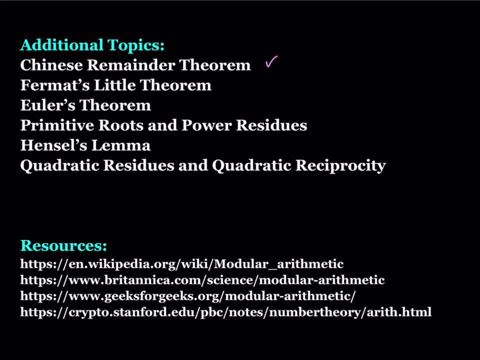 Firmly. I'm going to talk about a few other things, but first let's go over the others in this. Lemma's little theorem is very interesting, again for solving congruences. Euler's theorem is obviously huge, And then there's a couple other topics. There was one video that I made that could. 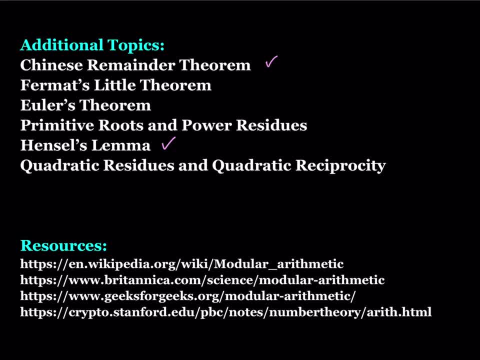 use Hanzel's lemma, Remember there was a mod 49,, I think, problem where you have the prime power modulus And those are very interesting topics And, of course, quadratic reciprocity is super duper interesting. And these are some of the resources that I used. I'm going to include these. 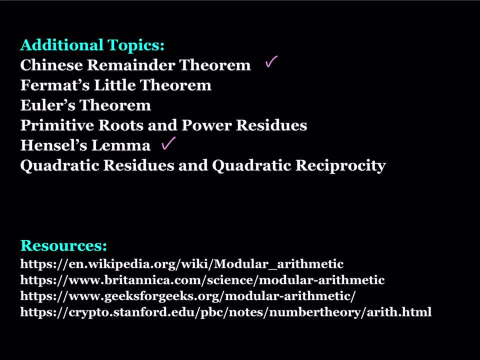 in the description as well. And one more time. this brings us to the end of this video. Thank you for watching. I hope you enjoyed it. Don't forget to comment, like and subscribe. Tomorrow I'll see you with another video. Until then, be safe, take care and bye-bye. 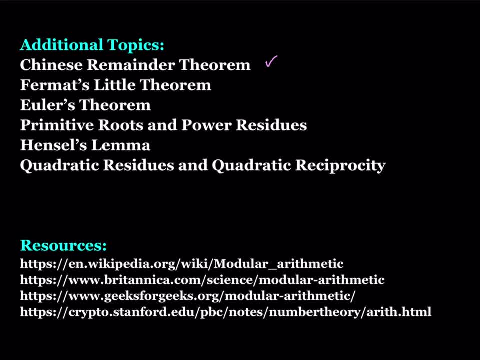 and for solving congruences. Euler's theorem is obviously huge. And then there's a couple other topics. There was one video that I made that could use Hansel's lemma- Remember there was a mod 49,, I think, problem where you have the prime power modulus And those are